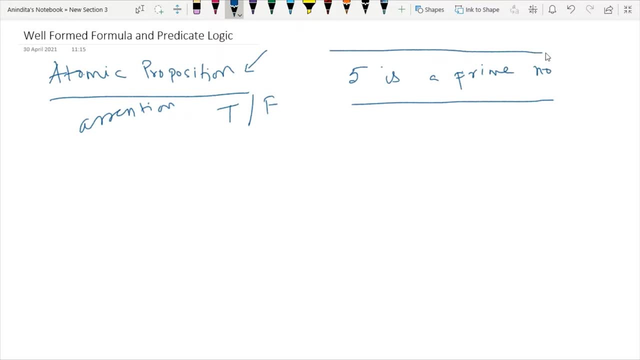 proposition because this particular statement has one particular true or false assertion 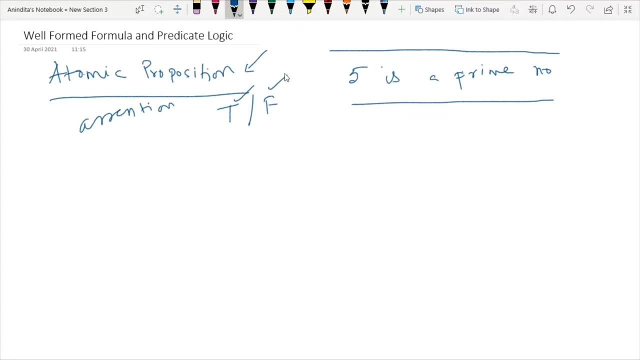 so now propositional formulas are constructed from this atomic propositions by using some logical connectives now what is the definition of propositional formulas propositional formulas are created by using this atomic propositions with propositional formulas some logical connectives just like and or implication something like this so if i write 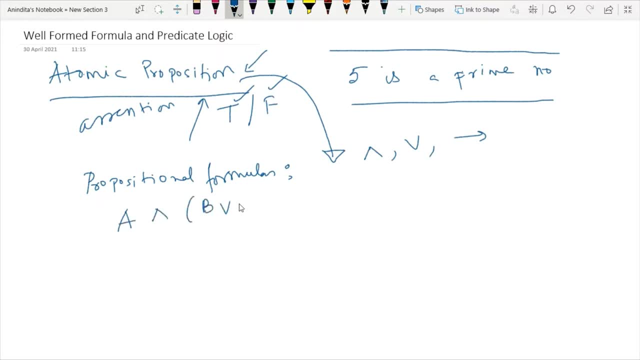 a and b or c implies b i can state that it is a particular propositional formula because this formula is constructed by using some atomic formulas which are connected via some specific connectives so my point is try to understand here a means we can assume that a is holding some particular english statement 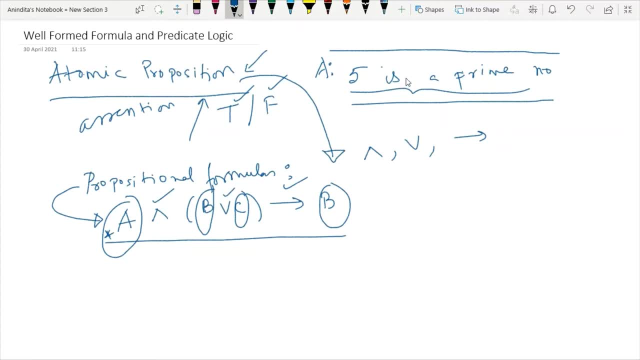 more precisely a is holding some atomic formulas so what is the definition of the propositional formula propositional formula is something that can be constructed by using some specific connectives and they are constructed by using atomic propositions and they are connected via some logical connectives 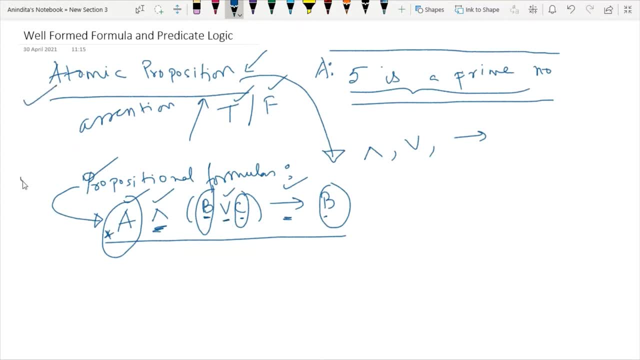 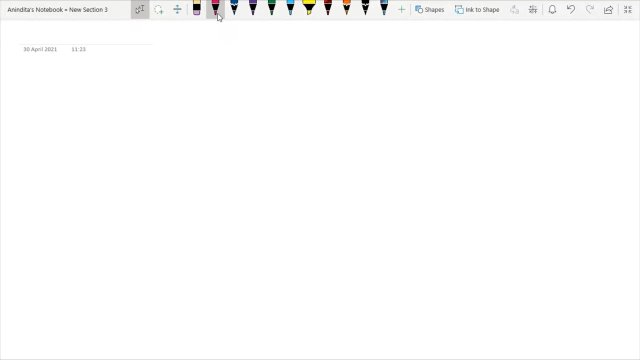 so in the previous class these are the two topics that i was discussing now today i am going to discuss the concept about well-formed formula first i will give you some rules at this point of time it is not easier for you to understand these rules but later I will give you example for each and every rule. So to understand the concept of well-formed formula that is WFF we have to extend our concept from 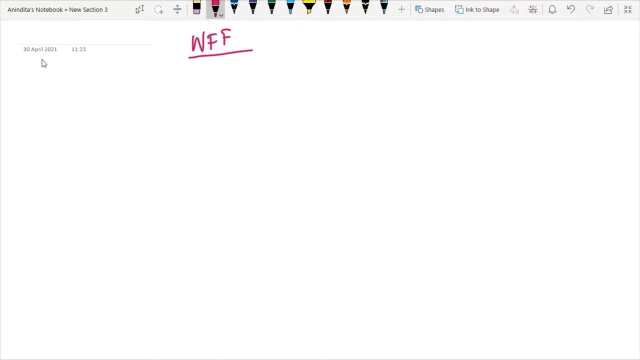 the atomic formula or atomic proposition. So I can state that the well-formed formula of propositional logic are obtained by using some construction rules. Now what are those rules? The first rule is an atomic proposition is a well-formed formula. So whenever you have any atomic proposition you can state it as a well-formed formula. So the rule number one is an atomic proposition. 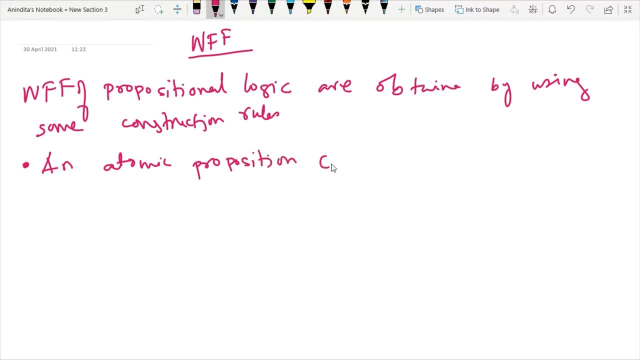 Say phi is a well-formed formula. Now rule number two is if you have one particular atomic proposition that is phi we know that it is WFF any atomic proposition is WFF. Then we can also state that not phi is a well-formed formula. So if you have one particular atomic proposition that is phi. Is also WFF means. 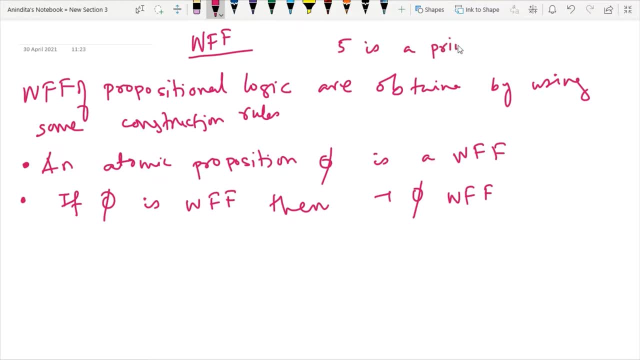 If phi means this one. So in this case phi is a prime number is a atomic proposition. So we know that according to rule number one it is by default WFF. However if I write phi way. 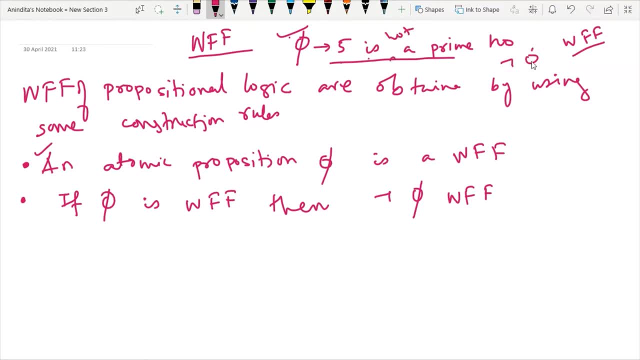 not a prime number then I will write not phi. So in that case not phi is also a WFF. This is your 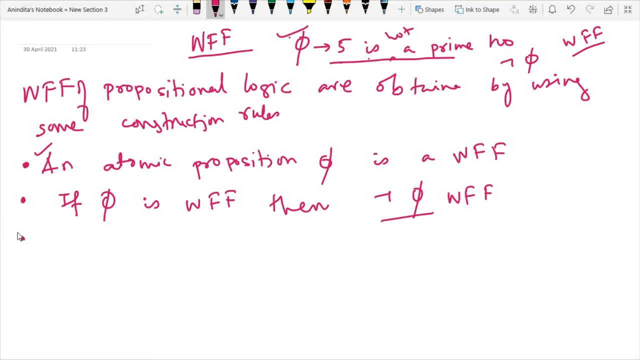 rule number 2. Now what is your rule number 3? So from this rule onwards we have to understand the concept of WFF in more details. According to rule number 3 if phi and theta are WFF. 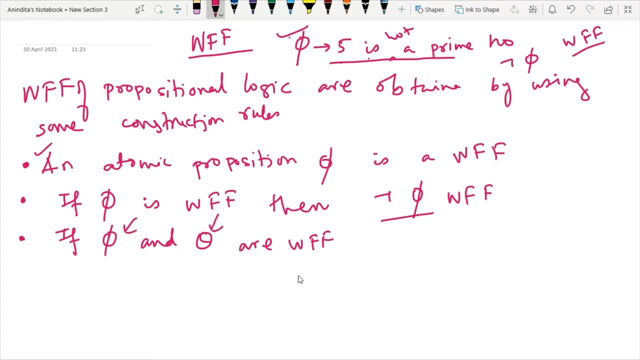 So if we have two statement which are known to be WFF then we can say that phi and theta is a WFF or phi or theta is a WFF. 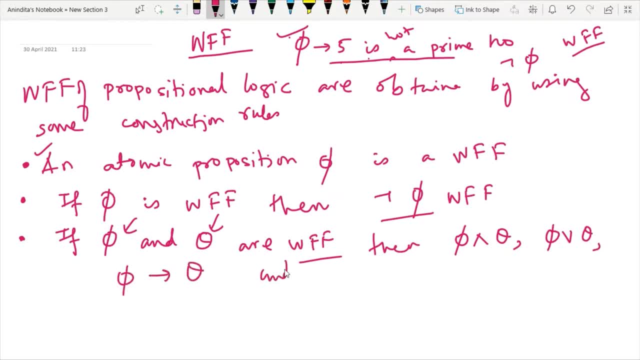 Or phi implies theta and phi equivalent theta which is also WFF. What is the meaning of this statement? I will explain it later on. Now your rule number 4 it is also difficult 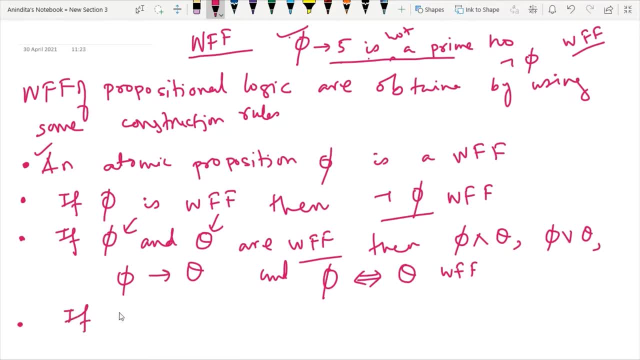 to understand that is if you have a particular variable x. So if x is a variable which represents some object of the universe and phi is a WFF then we can state that for 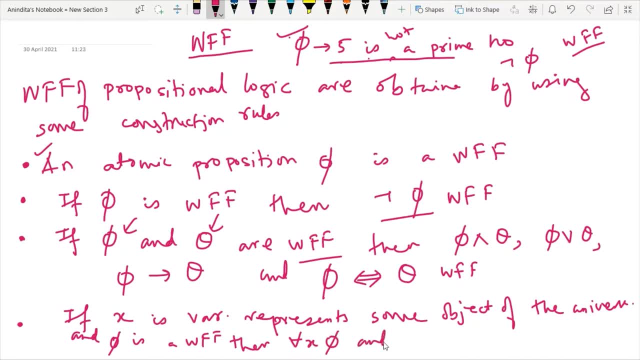 all x phi and there exists x phi is WFF. 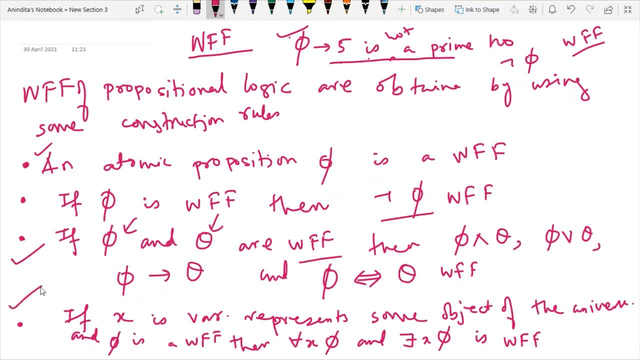 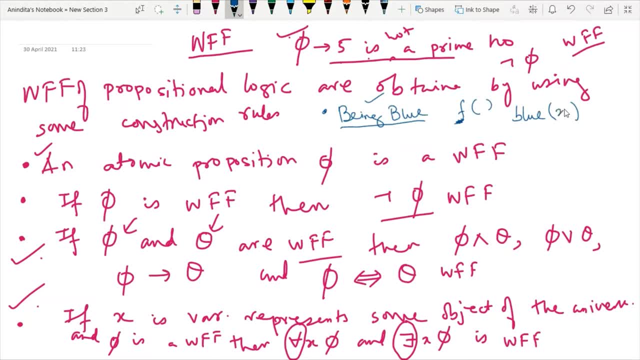 so in that case we will use some variable so in that case i am writing blue x the meaning of this line is x is blue so in that case the question is is it a wff this is the first question so x is blue is a atomic statement and we know that according to rule number one definitely it is 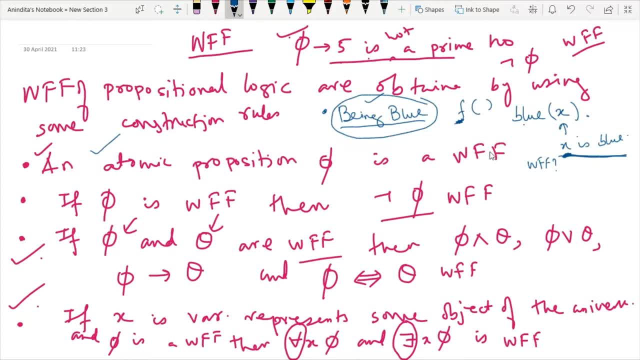 wff now consider another example say if i want to write that all x are blue 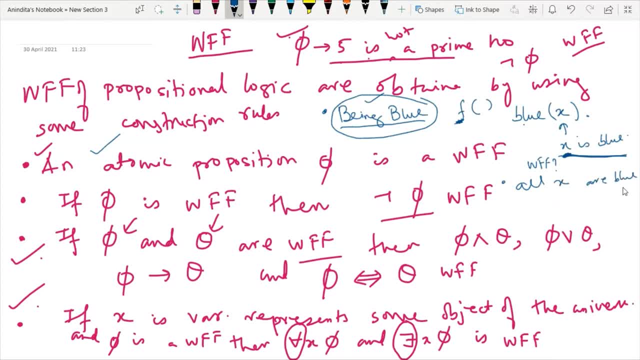 so how could i represent this so whenever we have the concept of all everyone someone in that case we have to use one particular quantifier which is known as all that is this symbol to mention for all we have to use this quantifier afterwards all x so for all x the statement is x is blue or x are blue so whenever we have all so we have to write x are so how we can represent this x is blue and x are blue both are the same concept so i will use the representation as blue x so meaning of this portion is for all x and meaning of this portion is x is blue or x are 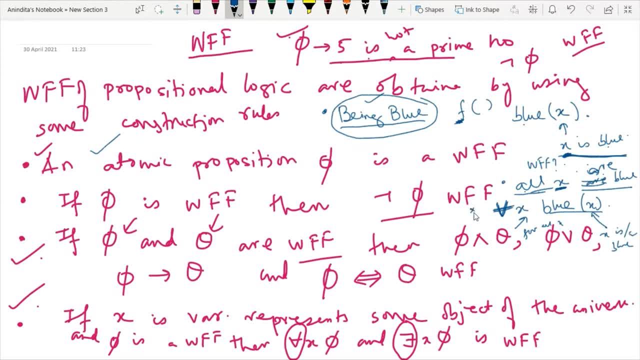 blue so in this case the question is is it a wff my answer is yes because we know that x is blue is an atomic formula so whenever your phi is an atomic formula it is itself known as wff and whenever we use this kind of representation for all x and then one atomic 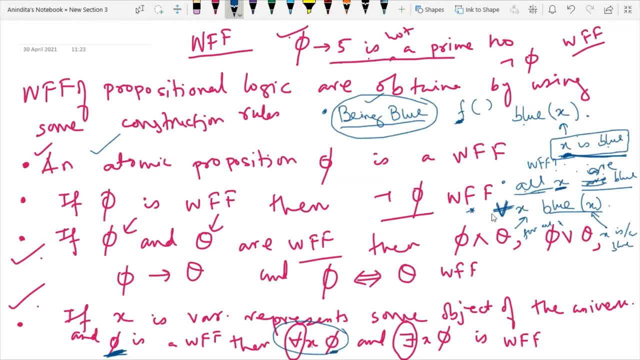 formula then it is also a wff so here i have used this representation for all x then the atomic formula that is the phi it means for all x blue x is your wff similarly if i have another statement that 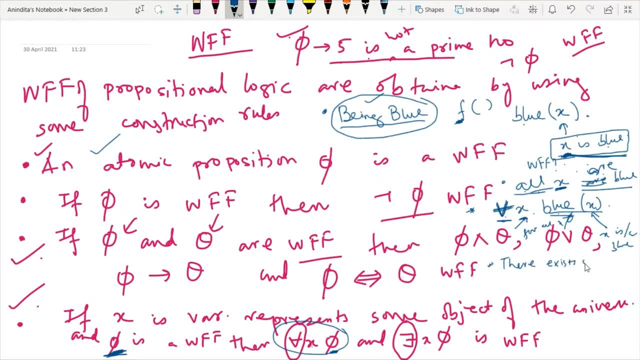 there exists some x which are blue so in that case how could i represent it so it is very simple there exists there exists to represent the concept of some there exists i have to use a quantifier 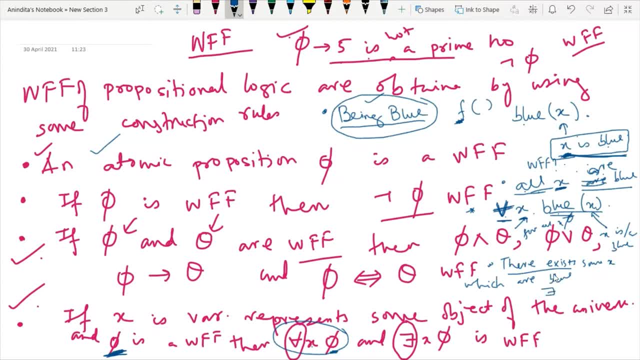 this one so this is a there exists symbol so for there exists some x so there exists x what is the line so some x are blue so in that case i will use the same concept blue x so here the meaning of this line is some x are blue so try to understand one point if the statement is given as some x are blue in that case also your representation will be for representing some x i will write there exists 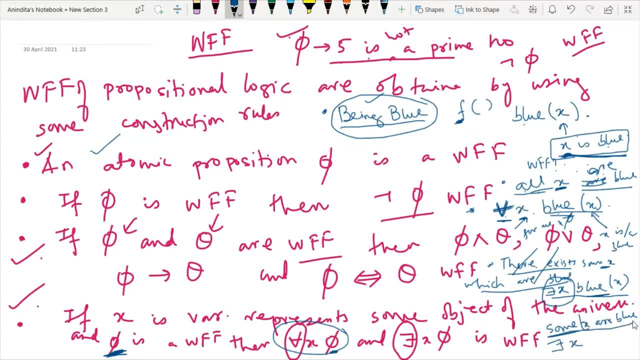 x and then for this line x are blue i will write blue x so now the question is is it a wff again the same solution if phi is an atomic formula for our case blue x is phi and whenever i am representing something in this manner there exists x and then the atomic formula it is a wff so there exists 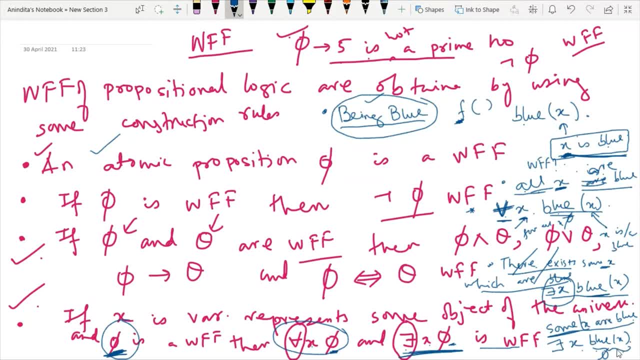 x blue x is wff so my point here is whenever you find any particular atomic formula or any atomic formula which has quantifier before it with some variable either this kind of quantifier or this kind of quantifier then the entire representation will be your well-formed formula 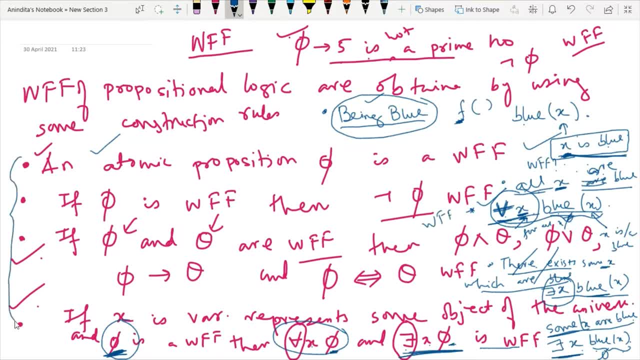 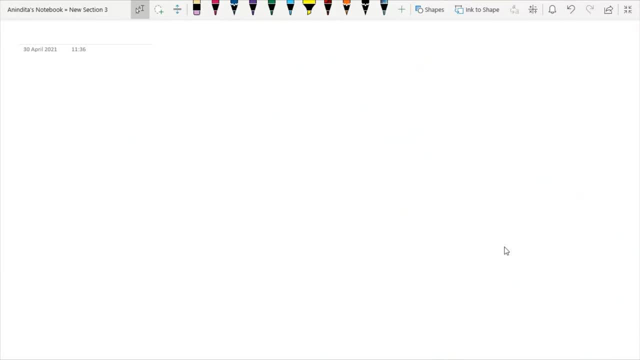 so these are the specific rules that is applied to construct well-formed formula now i will discuss one more point that is we know to construct wff we have some construction rules 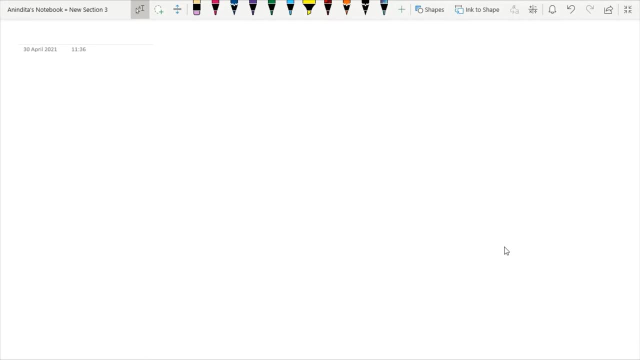 now i will mention another implicit rule i can say that each propositional constant constant and each propositional variables are wff so now try to understand this rule means whatever rule 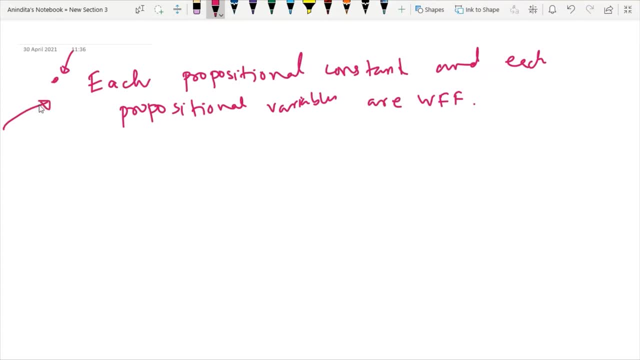 we have studied from that rule one implicit rule is also derived each propositional constant and each propositional variables are wff 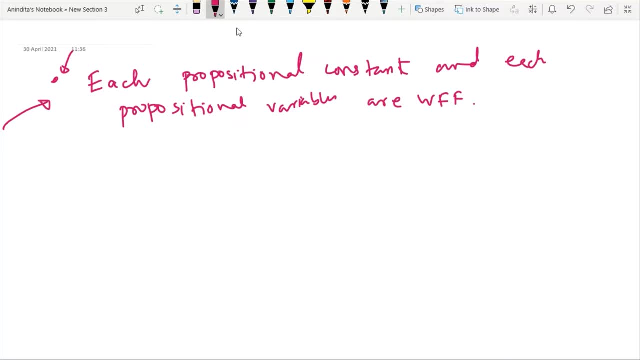 now what is the meaning of this rule i am giving you another example say the statement is written as the capital of india is new delhi say this is the statement so how could i represent this so in this case try to understand representation i can write 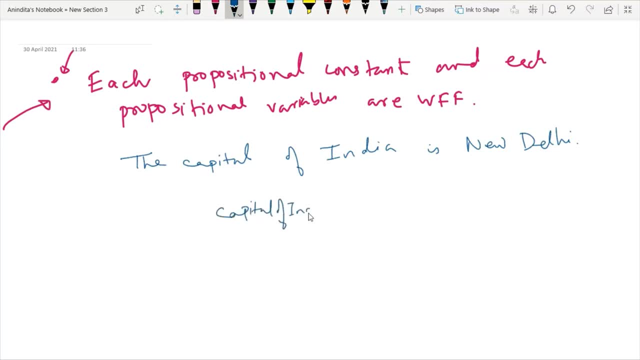 capital of india this kind of function name i can use and then i can here write new delhi so here i am not talking about the representation here the point is each propositional constant and 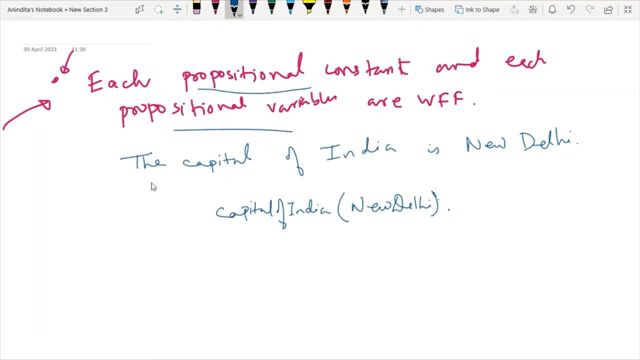 each propositional variables are wff so whenever you find this kind of line so this line is definitely wff , 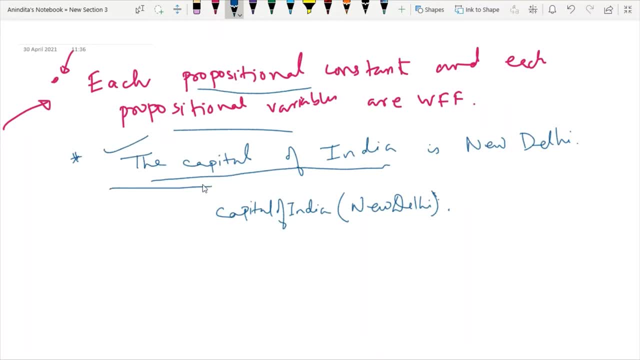 best reasonable distribution Bohr and this atomy statement here 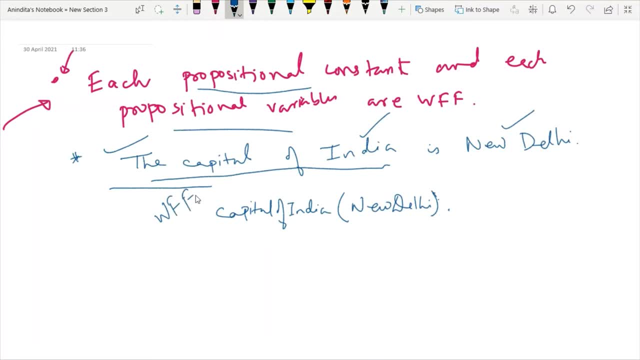 we are using some constant something. thing thing 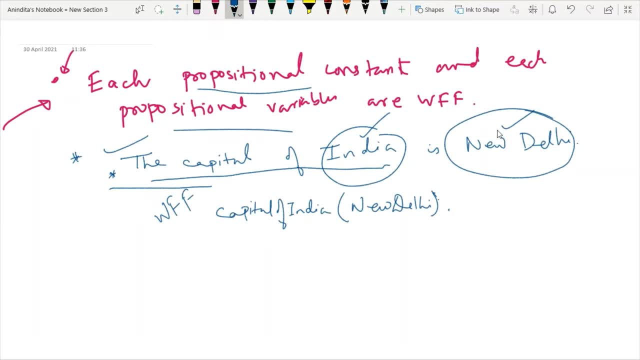 two terms as combo , one part 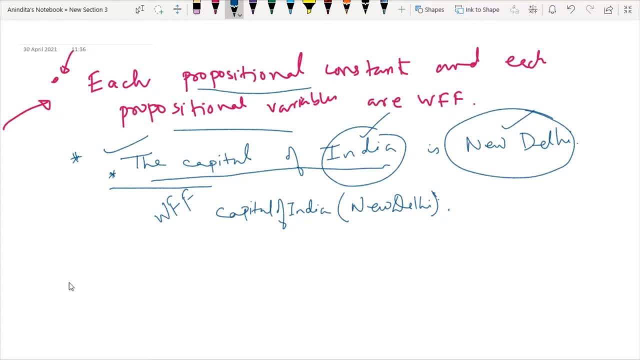 what are the rules of WFF so now consider this case we have studied that if we have two WFFs like this if we can write phi and theta or if we can write phi or theta these are also termed as WFF now we have to understand why say we have two atomic formulas that is x is blue and x is an atomic formula now how we can represent this so what I will do x is blue before the connective this is one atomic formula so and x is an atomic formula after the connective this is another atomic formula so here it is 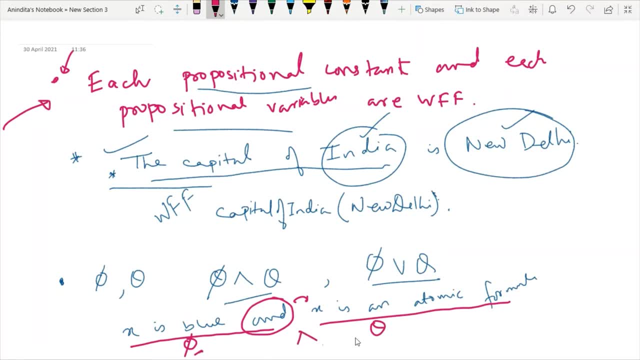 satisfy the third rule phi and theta so since phi and theta are atomic formulas and they are connected via connective and so according to rule number three we can state that this entire example is a connective and so we can state that this entire example is a connective 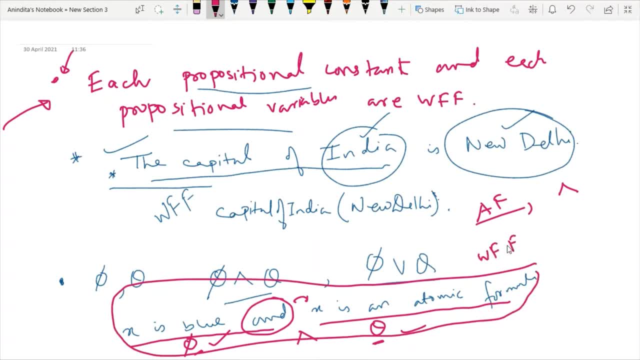 and so when we see here this is as if this eşapic formula so we will know that one is as simple as this one this is the we won't be using the знакомY 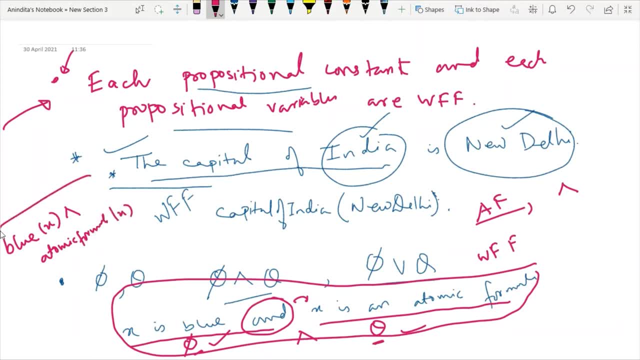 so two you know the thick and compassionate feels this is the thing called black places so i will write x becomes negative so the second example is WFF so what will be the representation so the representation will be x is blue the answer is yes. So here the question is is it a WFF the answer is yes this atomic formula phi is WFF this atomic formula theta is WFF therefore that it is blue. So here the question is is it a WFF and the answer is yes this atomic formula phi is WFF this atomic formula theta is W FUCK therefore there are too many examples here. 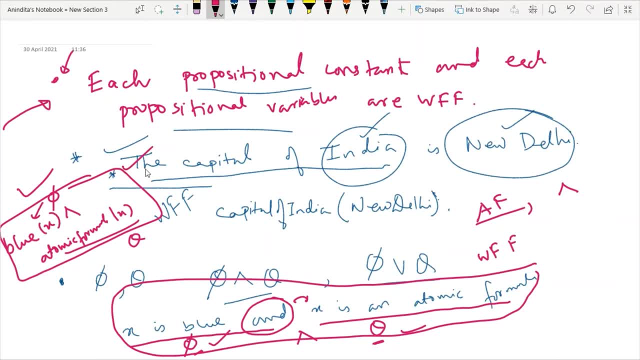 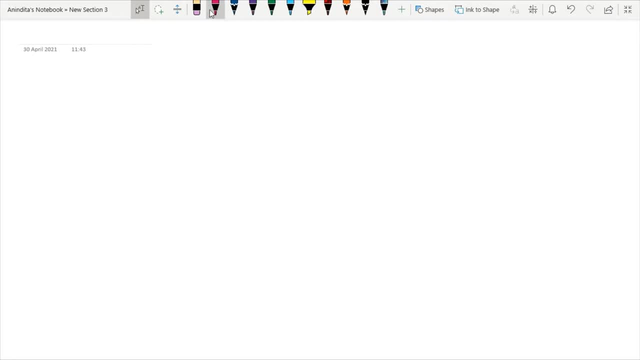 wff therefore this entire representation is also wff now i will tell you some other rules where you have to understand the statement which are not wff 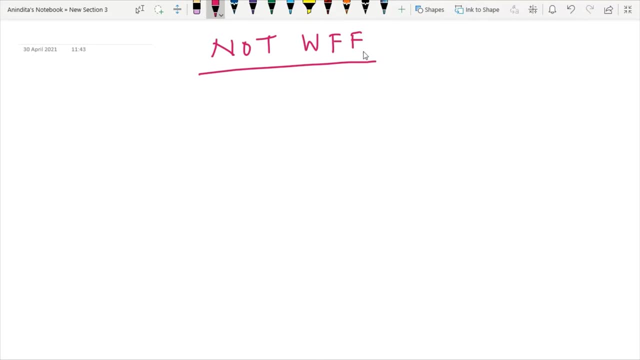 now i'm giving you some simple statement first say it is written that tom is taller than john so now how could i represent it in terms of function so i will write 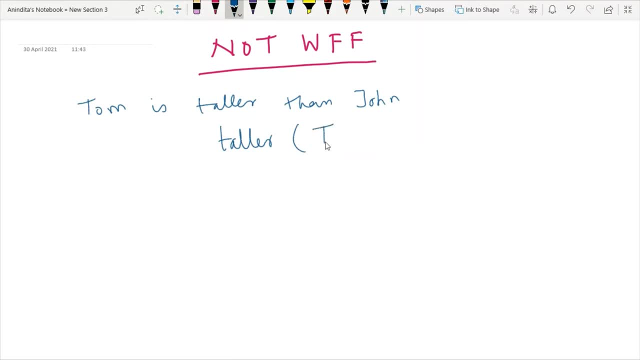 taller tom is taller than john so tom comma john 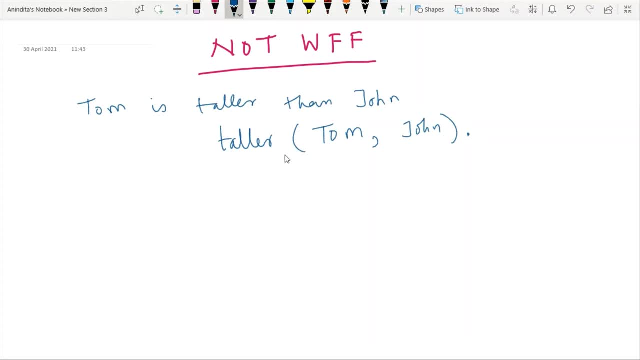 and you have to understand one more thing that i have to mention that each and every function is also known as fact representation and remember each and every fact representation ends with a dot so here I am intentionally giving this dot so what is the meaning of this statement Tom is taller than John now I 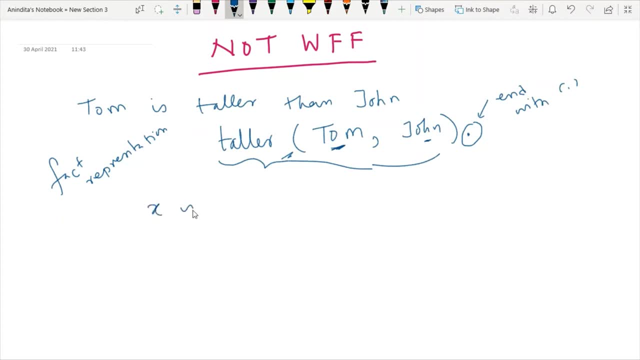 am just writing that X is representing people in the world means X is a variable so in that case if I have a statement that X is taller than Tom so in that case what should I write I will write taller who is taller than tom x is taller than tom so this kind of representation is also allowed 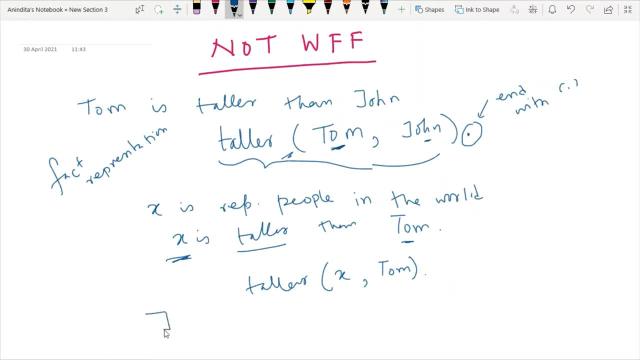 i may write that there exist x means some x is there for all y so the representation will be taller x comma y so the meaning is some x is taller than all y so this is the meaning of this line since the variable x is with the quantifier there exist it means some x is taller than all y because we have all quantifier with y 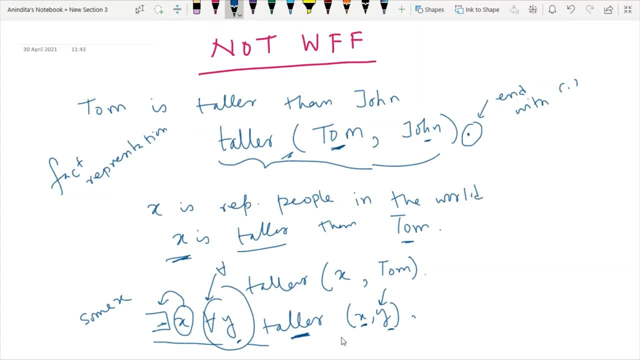 so this is the meaning of this statement now if you find some statement which is written as taller there exist x say john or tom something so at this point of time i will state you that this is not a wff because there exists 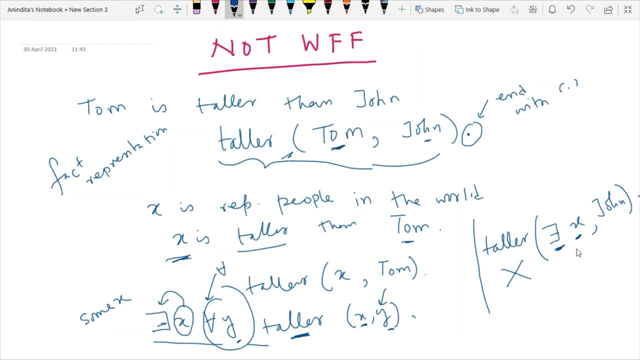 sign with the variable is not allowed as an argument inside a function in case of wff so this kind of representation is not a wff so i think you have identified this point whenever you are defining any function you can write constants you can write variable and constants as an argument or you can write two variables as an argument however quantified variables means variables with quantifiers 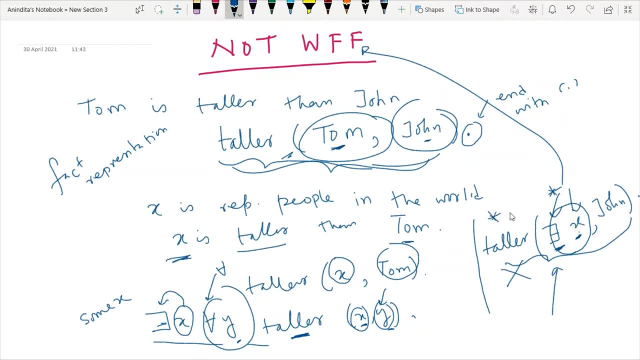 is not allowed as an function argument whenever it is written then straight away state that it is not a wff say i have one english statement written as and put that inside the url talk about it or so on familiarize yourself with an argument 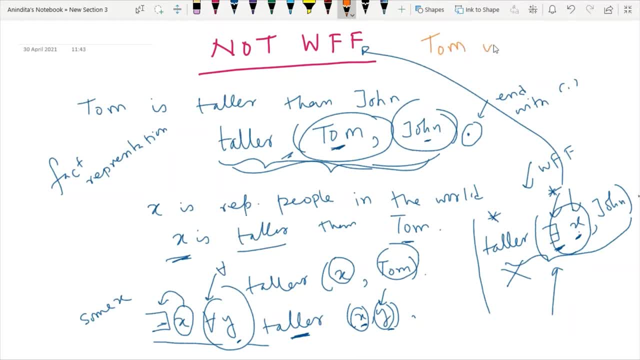 one english statement written as tom is not a man because we know that tom is a cat according to tom and jd cartoon so if this kind of scenario is there so i cannot write man not tom if 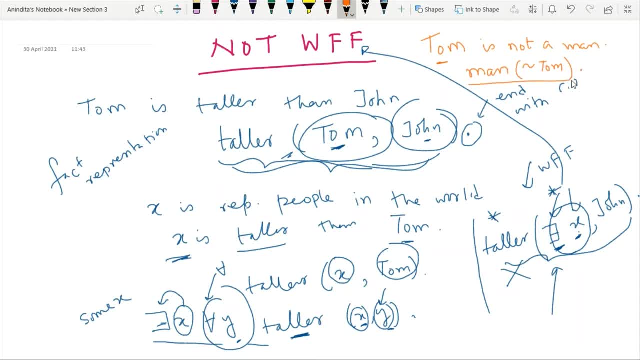 i use this kind of representation for representing that tom is not a man in that case it is not 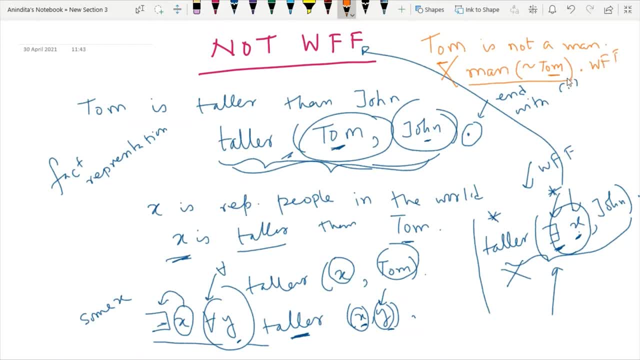 wff why in case of wff with the function argument not quantifier is not allowed so whenever you have not quantifier with the argument inside a function then it is also not a wff so so 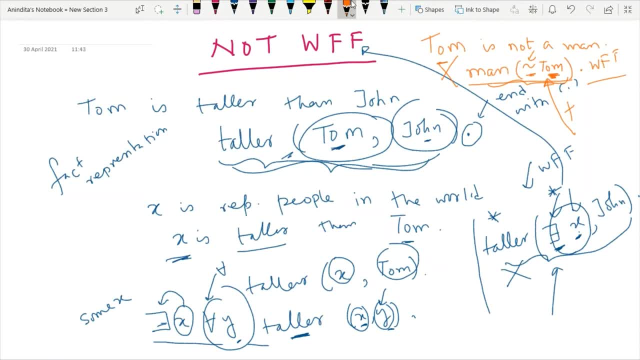 now definitely you will ask me this question so how could i represent this kind of statement so for that purpose we will learn some of the conversion techniques and we will learn some 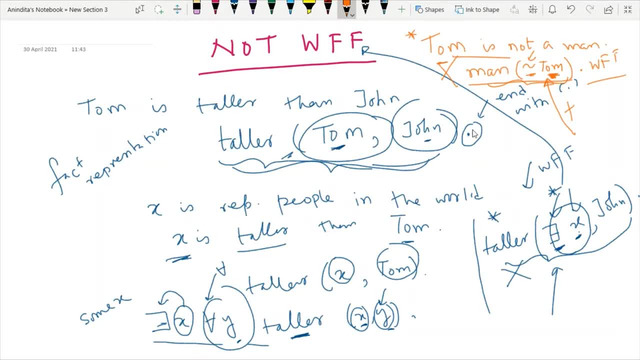 of the tips and tricks but here my point is which functions are not wff you have to remember i will tell you one thing that whatever we are studying it is known as fopl fopl 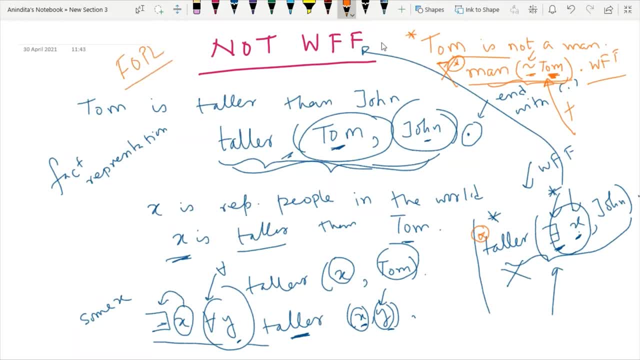 means first order predicate logic and whatever rule i have stated at this point of time since this kind of syntax are not supported in first order predicate logic that's why this particular 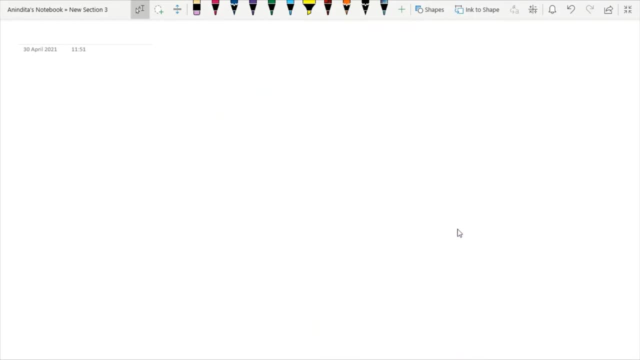 rules are not supported by wff i know there will be one question that what is the concept of predicate logic 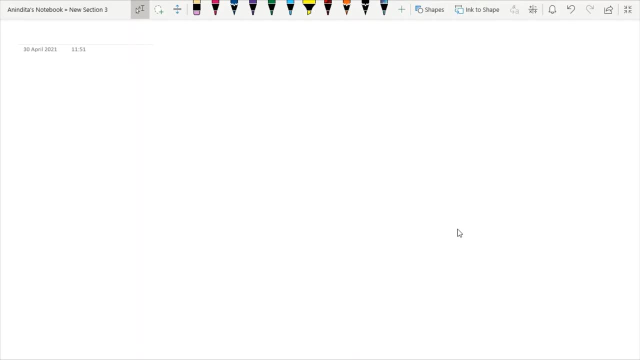 because when we use predicate when we use proposition we have to understand now i will give you one simple example say we have one english statement like x is an integer now why i am incorporating the concept of predicate here i will tell you we know that 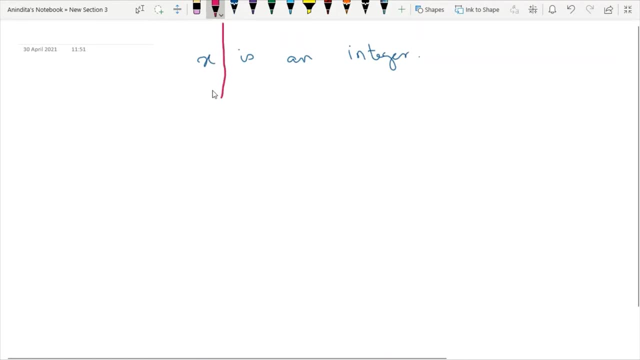 if i divide this statement into two part then x will be the subject of the statement and the second part will be treated as predicate so from this concept we will extend our mathematical predicate logic 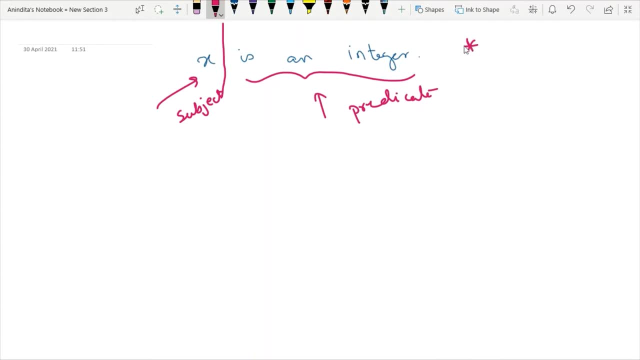 concept so now you have to remember one more point whenever we are using the concept of predicate then it is evitable that before your variable you might encounter with some words like all some this kind of words will be definitely coming so in that case remember one point predicate logic representation will use quantifiers and we have only two quantifiers 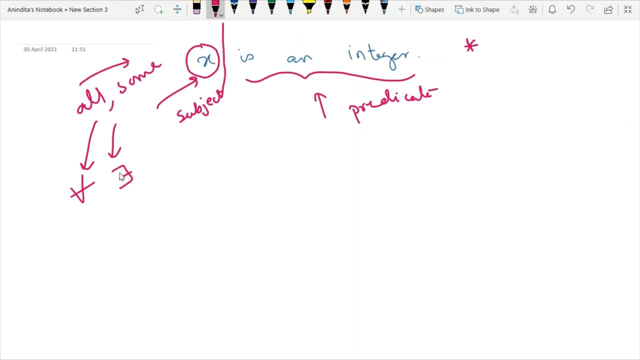 so what is the definition of a quantifier so what is the definition of a quantifier 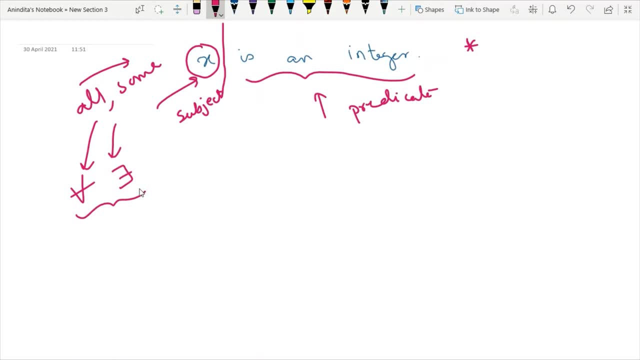 i can see that quantifier is a language element so i can treat them as language element that generates quantification quantification specifies the quantity of the specimen in the universe of discourse so my point is whenever i write for all it means it is representing for all 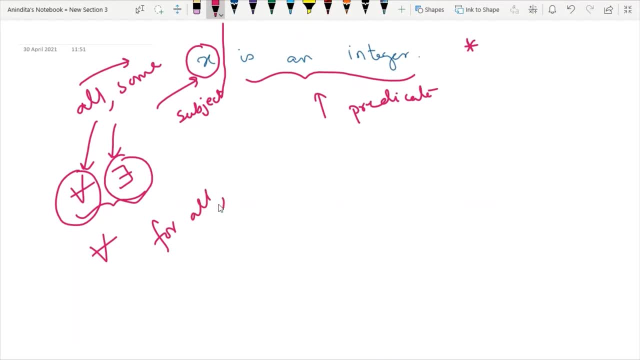 some quantity of the representation that exists in the universe or it will represent every one or it will represent everything so whenever we have this kind of words i can straight away use this kind of quantifier so it is a quantification thing and also whenever you find this quantifier there exists quantifier name of this quantifier is existential quantifier 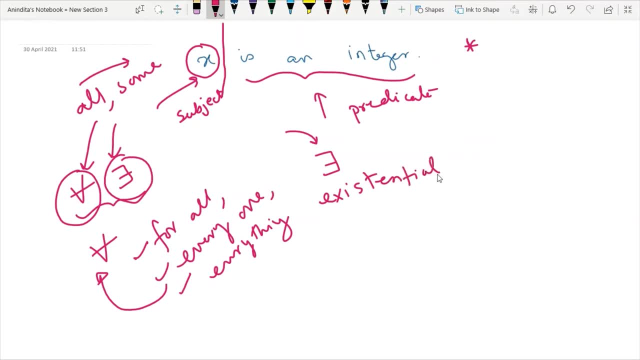 this existential quantifier represents for some at least one this kind of quantity so definition of the quantifier is it is an language element that 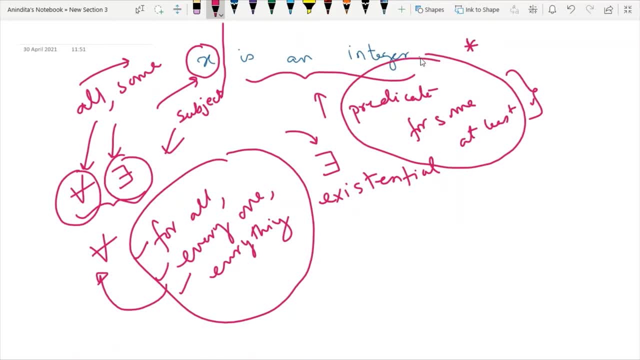 represent quantity of the universe of discus maybe some maybe all so this is a quantification thing so that's why we will use the quantifiers so predicate logic comes with 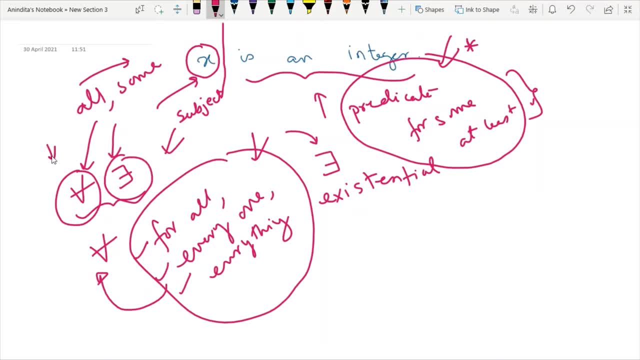 this quantifiers however whenever we did some problem in the previous class using propositional logic there is no question of quantifiers so my point is this is the biggest drawback of propositional logic that if a particular statement comprises of this kind of words 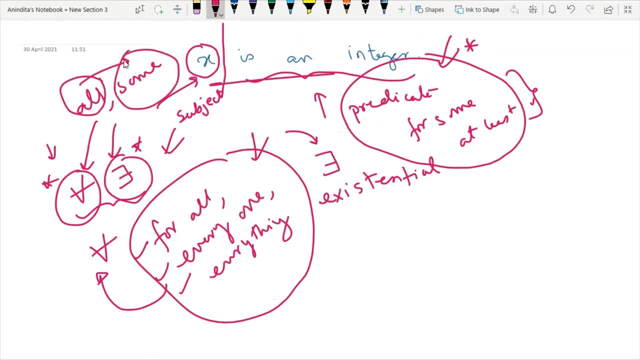 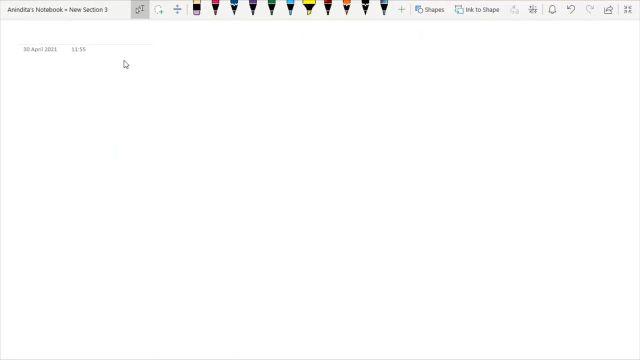 then propositional logic will not be able to represent so this is my point now we have to understand how could we represent any English statement with quantifiers and into predicate logic representation so now I will give you some example so first I am writing one particular 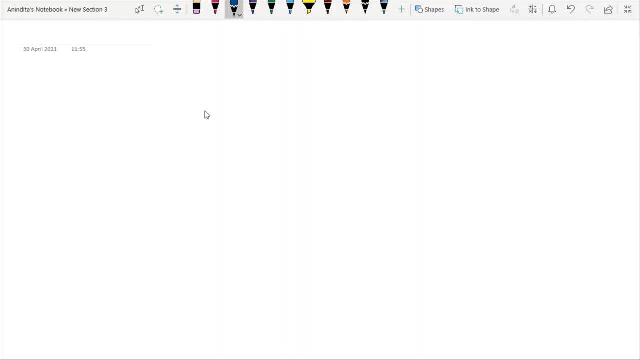 representation and how I am representing or how I am reading this line you have to understand so whenever I write this 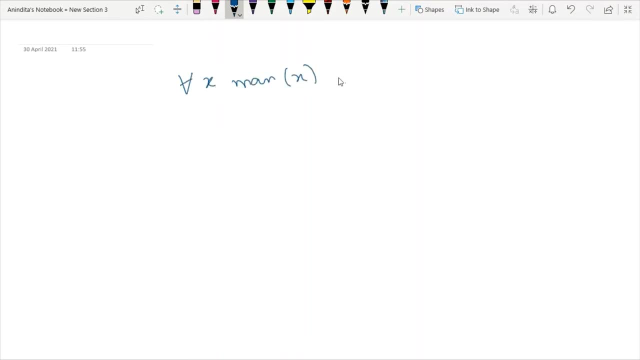 kind of representation. Now how I am reading it try to understand. Here the meaning of this segment is there are all X meaning of this segment is where X is a man who drinks coffee. 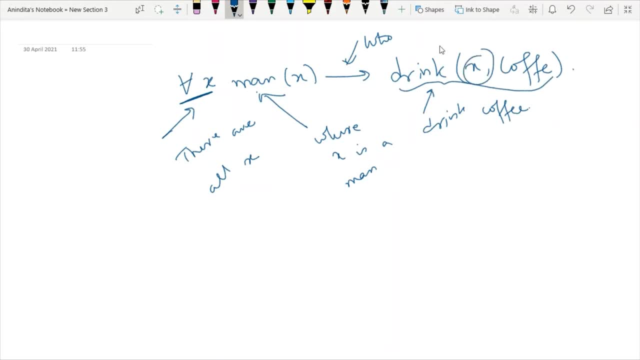 Hence the meaning of this line is X drinks coffee or X drink coffee. So try to understand how I am representing so there are all X where X means X is a man so I am talking about man person who drink coffee. So this is how we will read this kind of representation. 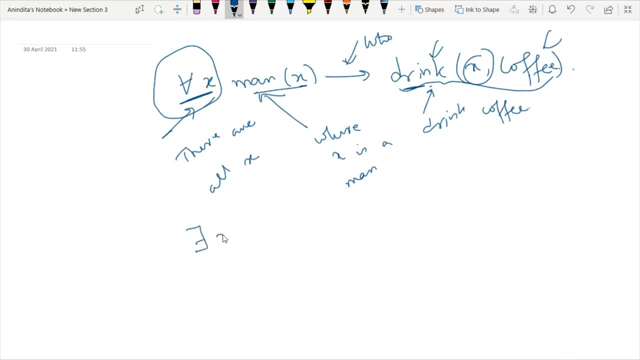 And now if we have this kind of representation there exist X boys X then one connectiv and then intelligent X. 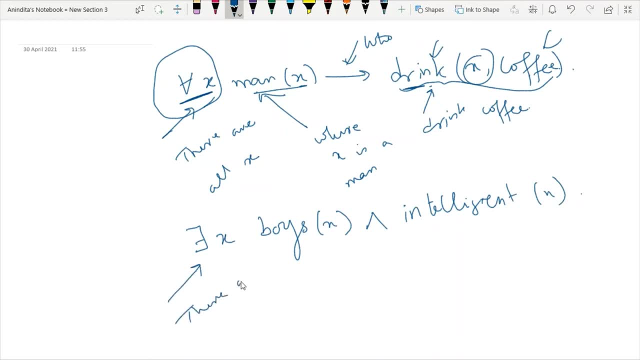 Now first try to understand how am I reading it. There are. Some X. Were X is a boy. So. 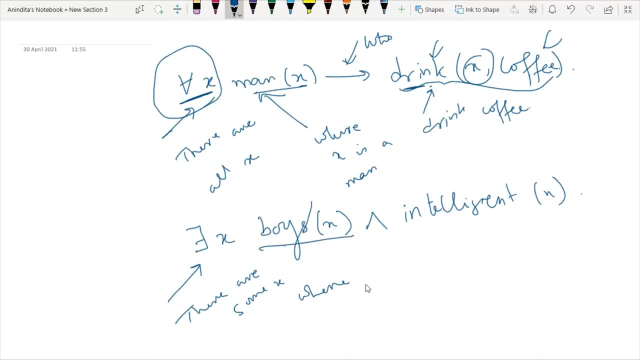 Here I can also write boy X where X is a boy. 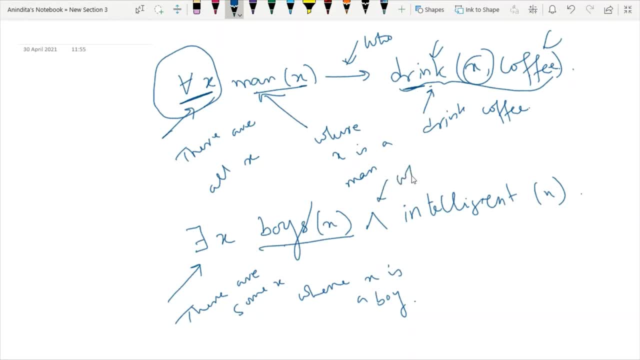 Who is intelligent? Who is intelligent? So meaning of this line is X is intelligent. 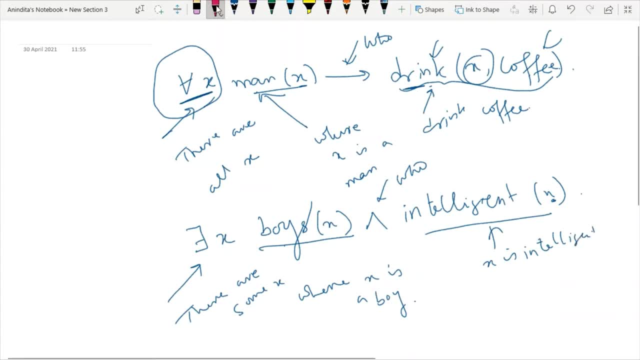 Now one question is very common. Whenever I am representing the term who. 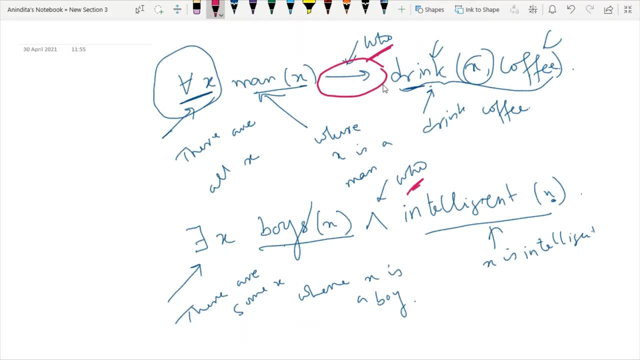 First I have shown implication symbol. In the second case I have shown one connective which is and connective. Now it is a kind of ambiguity I can say. 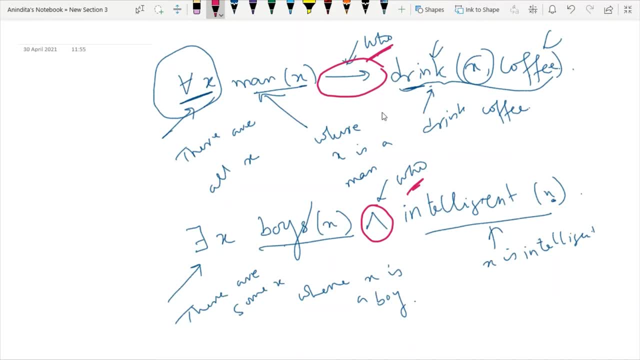 Because I cannot represent who with two different symbol. 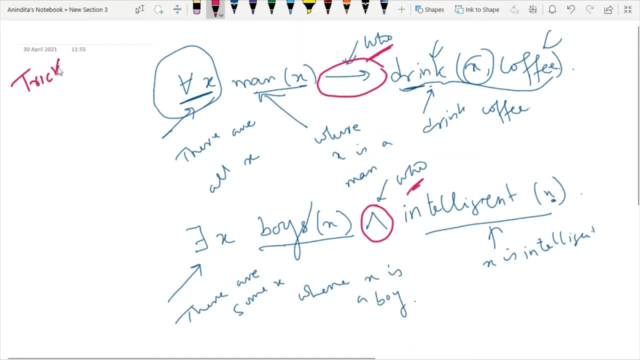 So here you have to remember one trick. The trick is. The main connective for universal quantifier for all is also known as universal quantifier. 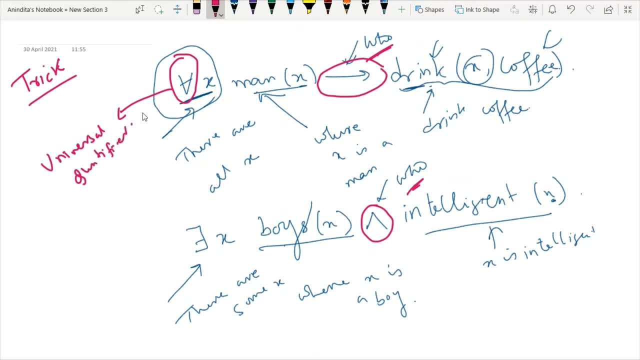 So whenever you have universal quantifier. The main connective that you will use that will be definitely implication sign. So implication will be the main connective for universal quantifier. 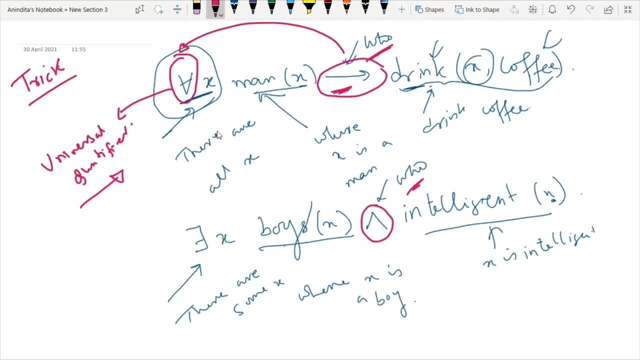 And now you can guess that for existential quantifier. What is the main connective? The main connective will be your and connective. 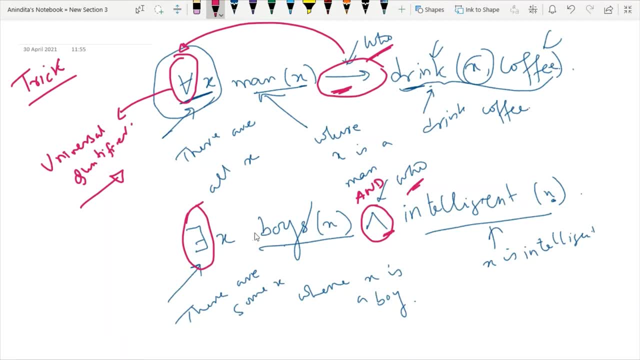 So the trick is whenever in your representation you have all. Definitely you will have implication sign as a main connective. On the other hand for existential quantifier you will have and connective. So this is the main connective. So this is the first trick you have to remember. 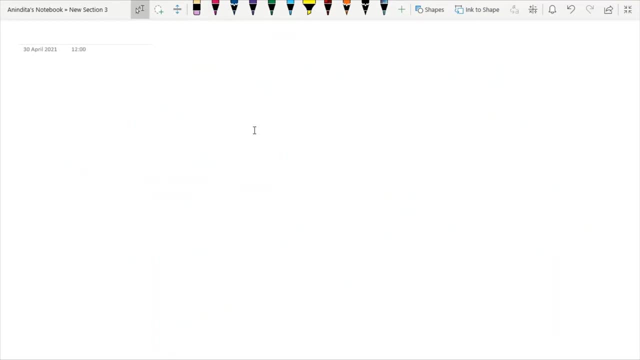 Now how we can represent a particular English statement. Now I will give you one example. Say our example number one is. All birds fly. 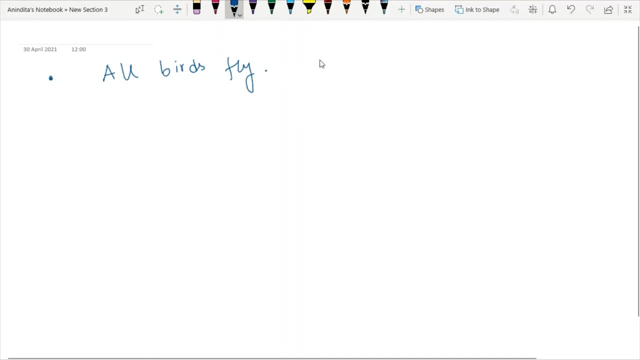 Now your first question will be. What kind of representation should I use? Should I use predicate or should I use proposition? So my answer is. Very clear. 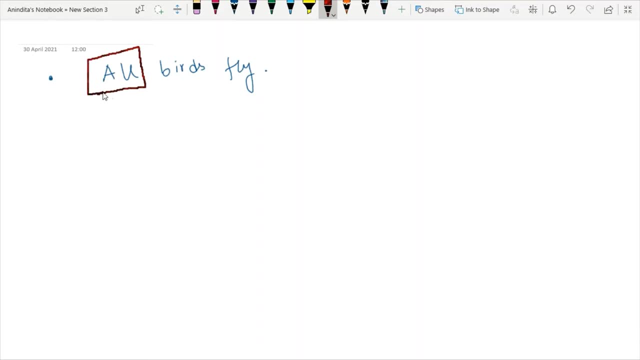 I have all word with my English statement. So to represent all I have to use universal quantifier. So whenever universal quantifier we are going to use. Then definitely our representation will be predicate representation. Now in case of predicate how could I represent? In case of predicate representation we will use some function. So what kind of function I can use? This is your subject and this is your predicate. 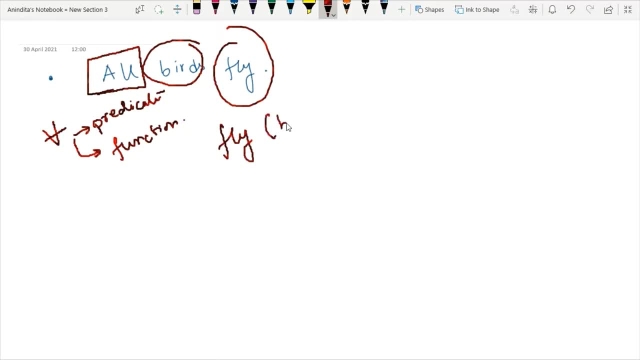 So in that case what can I write? Fly bird. 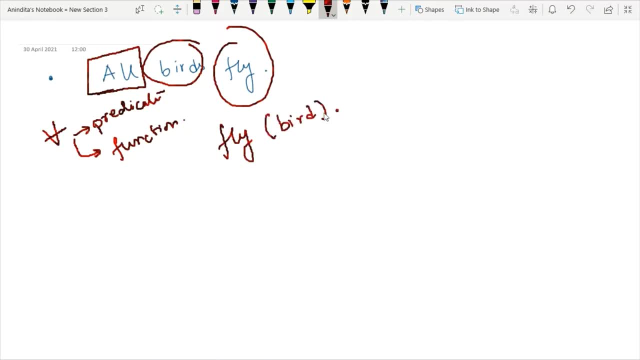 So this is the first step. So whenever you have any English statement. First try to find out. We need any quantifier or not. If we need any quantifier then definitely we can use it. 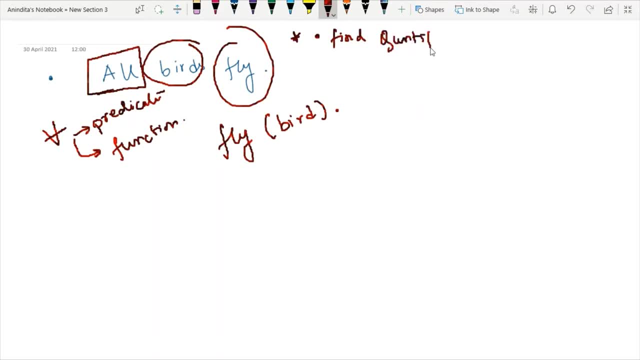 So whenever you have any English statement. First try to find out. 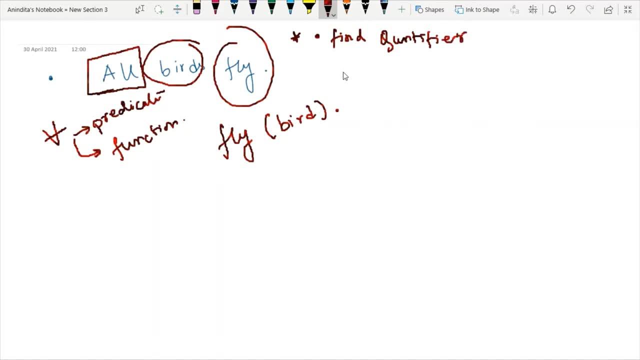 We need any quantifier or not. If we need any quantifier then definitely we can use it. 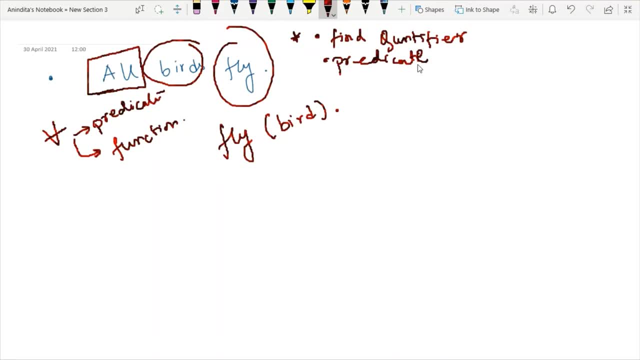 We can identify that it is a predicate representation. And then what you will do. You just divide the statement into subject predicate part. And just write the function. Now. 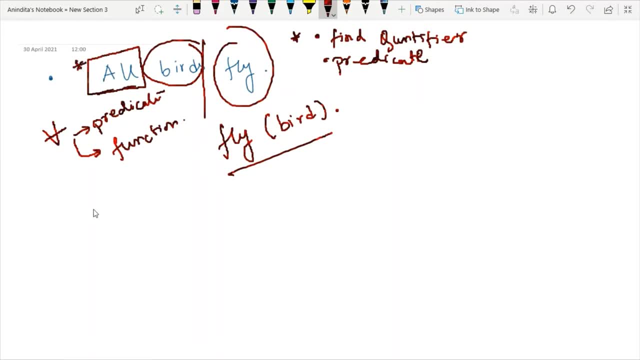 To represent the concept of all. For all x. 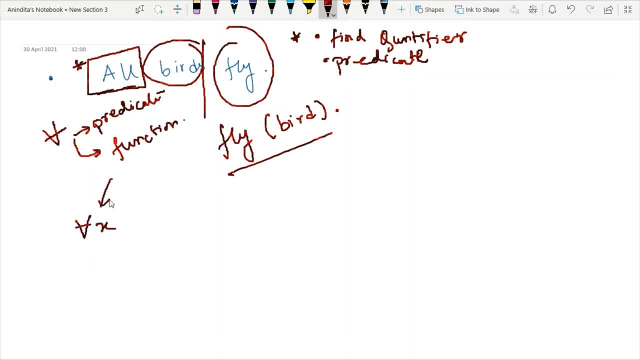 Means all bird can fly. So I am using here to represent all. All bird. 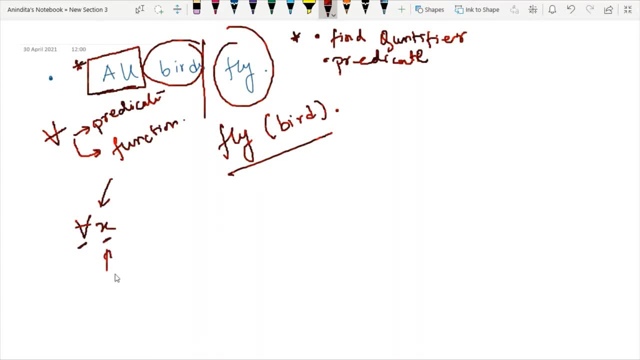 Means any bird. So for that reason I am using one variable. 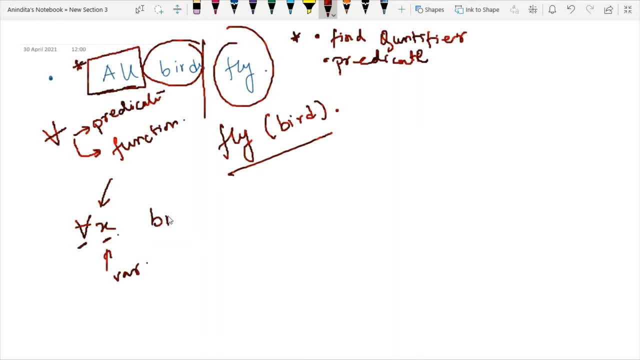 So all bird. Means any bird can fly. 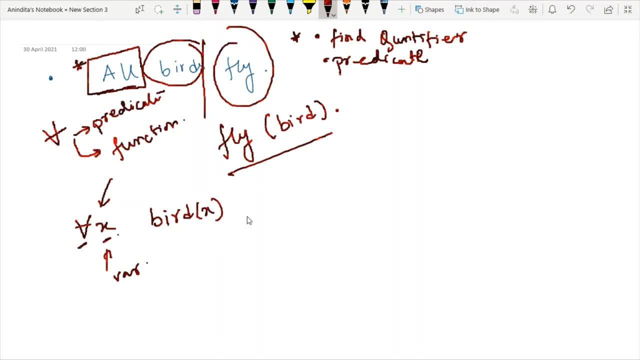 All x. Where x is a bird. 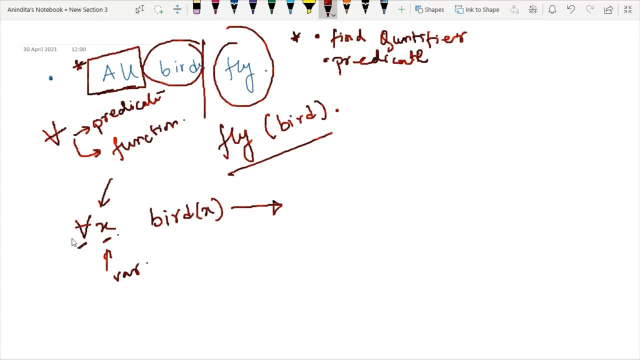 And here I have to use implication sign. Because we have. 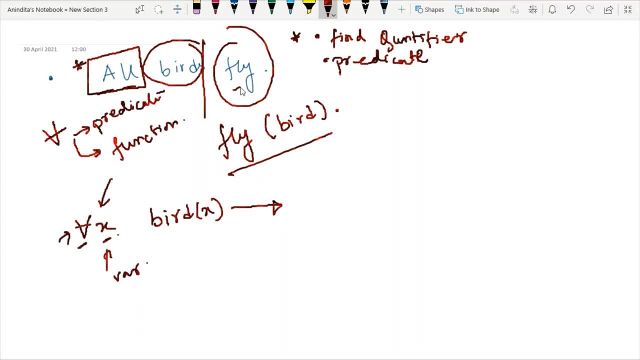 Universal quantifier. And the statement is. 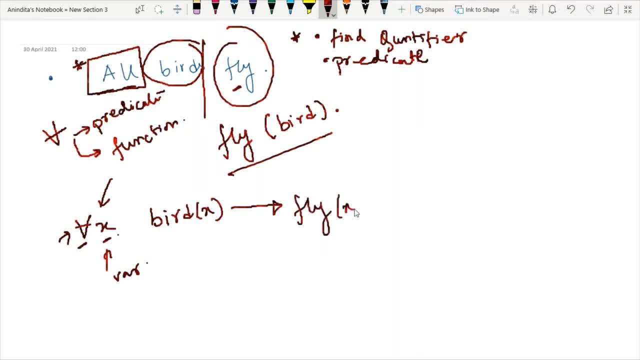 X can fly. So I will write fly x. 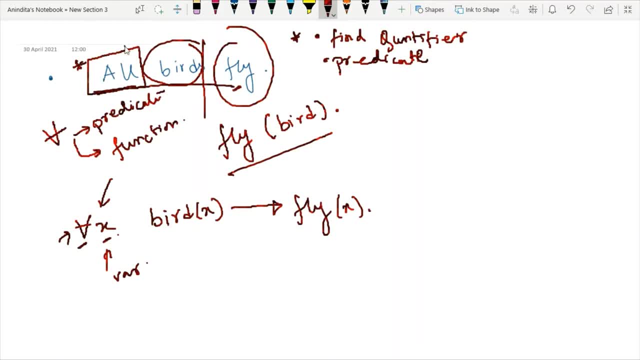 So what is the meaning of this statement? All bird. So to represent all. Means any bird can fly. 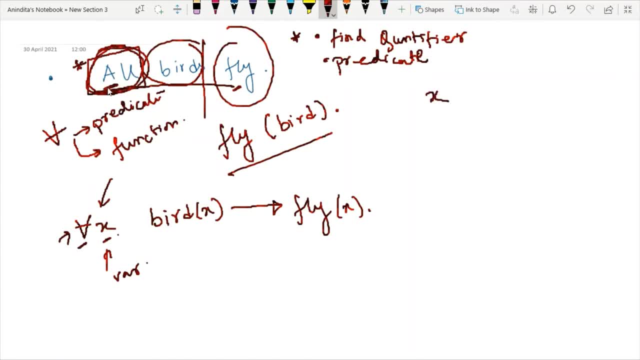 I am using one variable. For representing all. I am using this quantifier. And we know that. Whenever this quantifier is used. The main connectic will be. Implication sign. Now what will be the content of LHS. 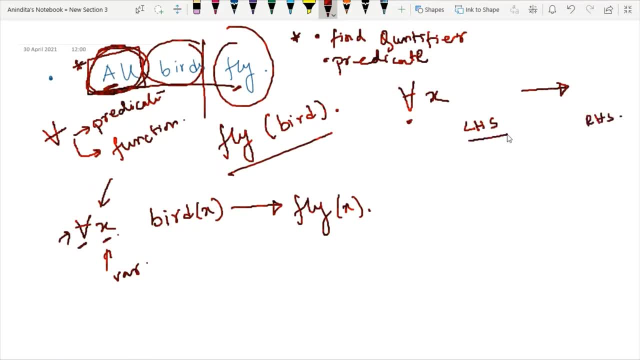 And what will be the content of RHS. So in the LHS. 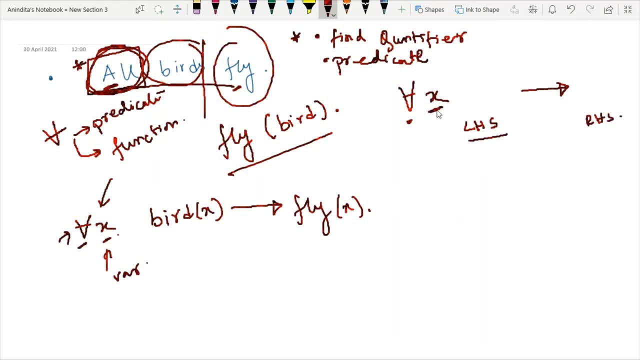 We have to define. What is the meaning of x. Because x is a variable. 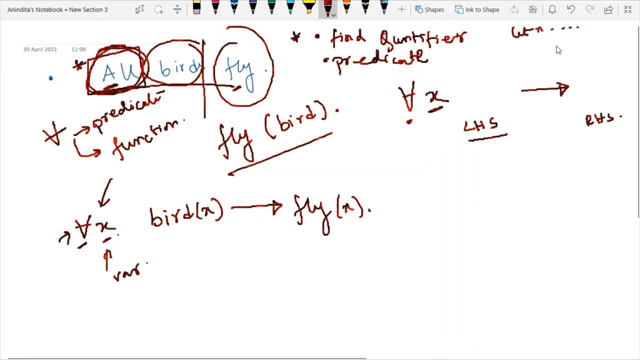 In maths also we have to write. Where x is something. Let x is something. So what is the meaning of x. 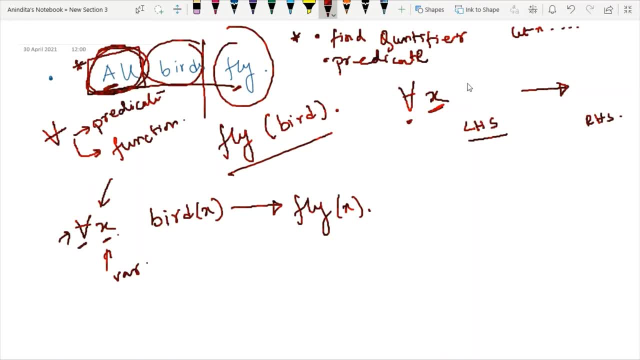 I am using variable x. To represent all birds. 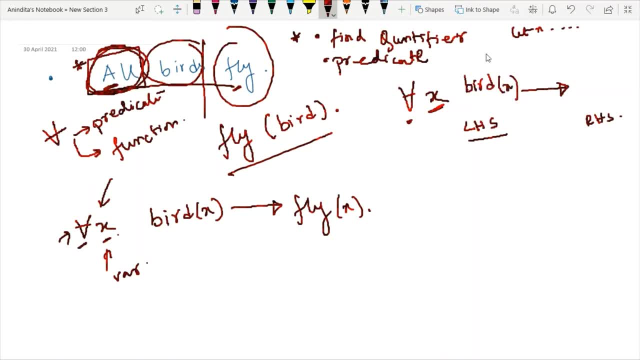 So basically my point is. X is a bird. 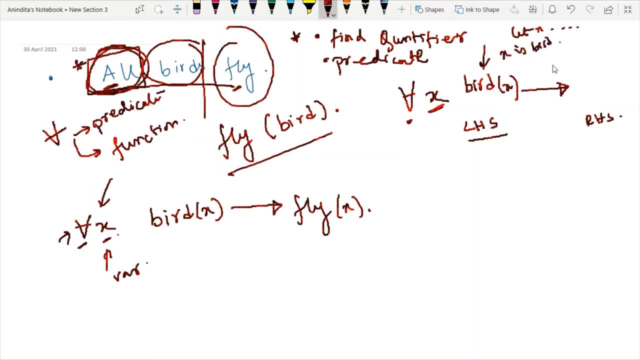 So meaning of this line is. X is bird. 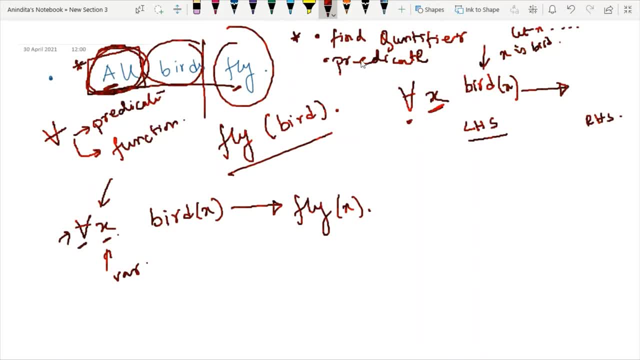 And in the RHS. What is the thing that I am going to represent. That bird can fly. 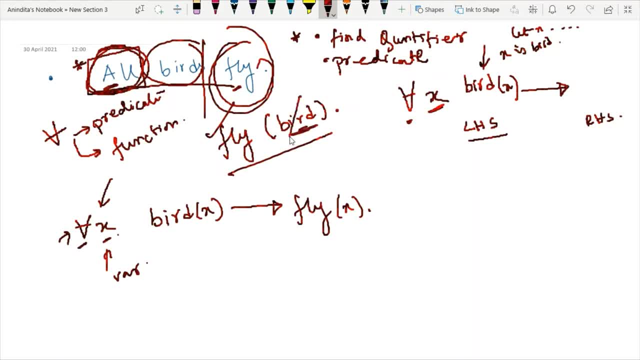 So here. This bird will be replaced by. The variable. That is fly x. 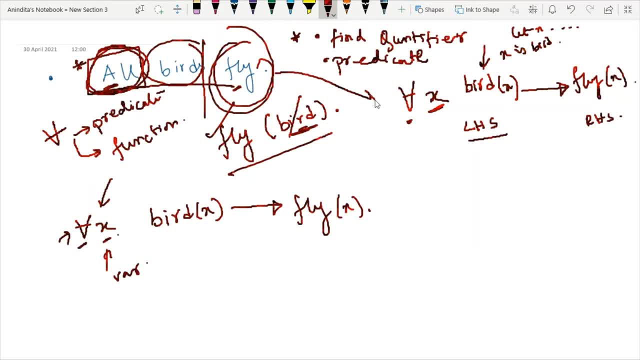 So whenever this line. Is given to you. Appropriate representation. Of this line. Now I will give you another example. So that you can understand it. Better. 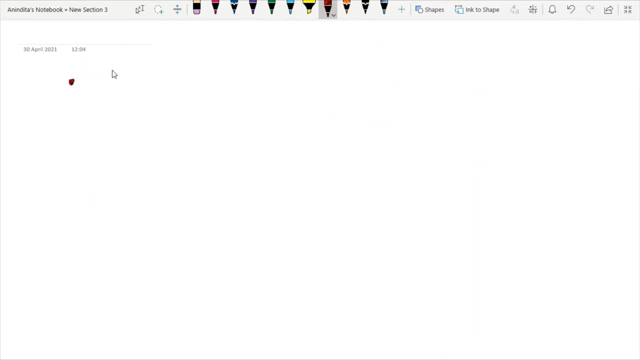 Example number 2. Say. The statement given as. Every. Man. Respects. His parent. 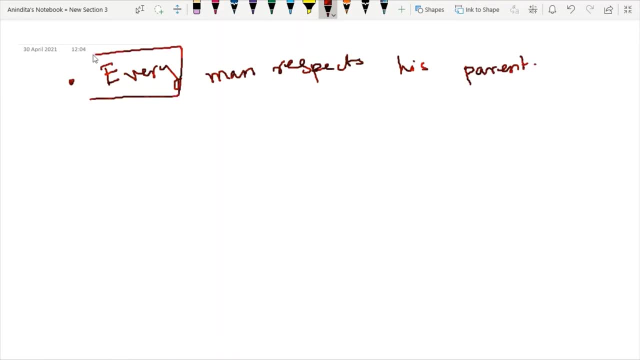 We know that. We have the word every. So for that purpose. I have to use one quantifier. 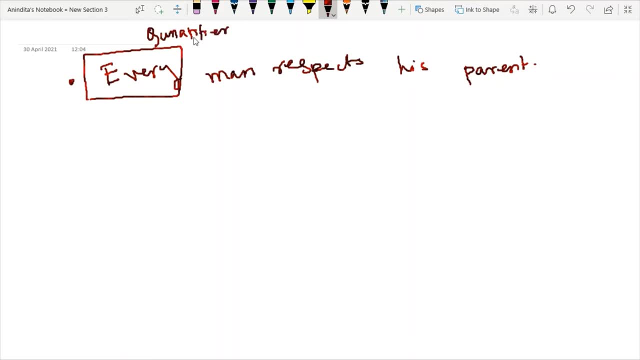 So using quantifier means. It will be my predicate representation. This is the first point. And then I have to identify. The function. 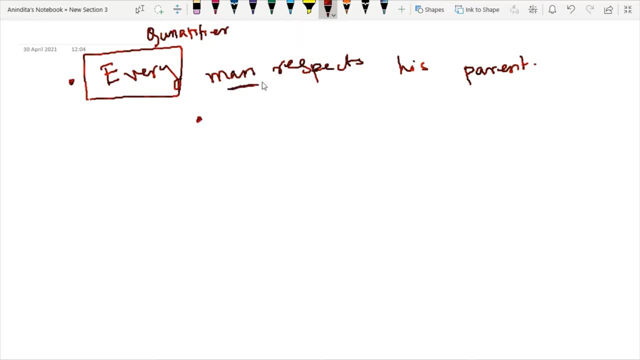 What I am going to represent. So basically my point is. 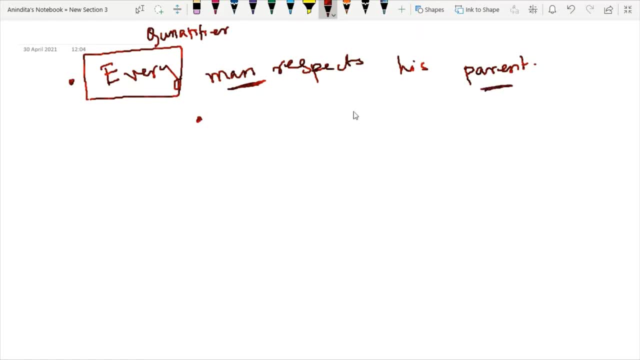 Someone. Respects someone. Right. 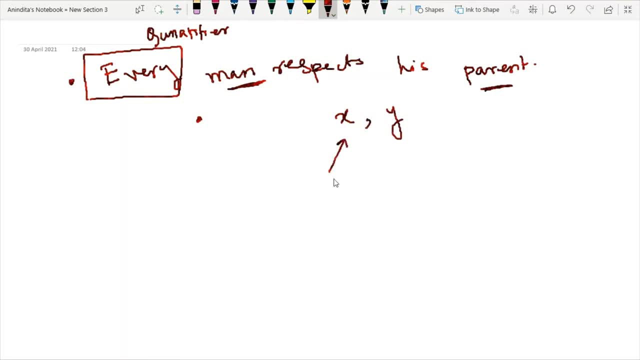 Someone. So my point is. 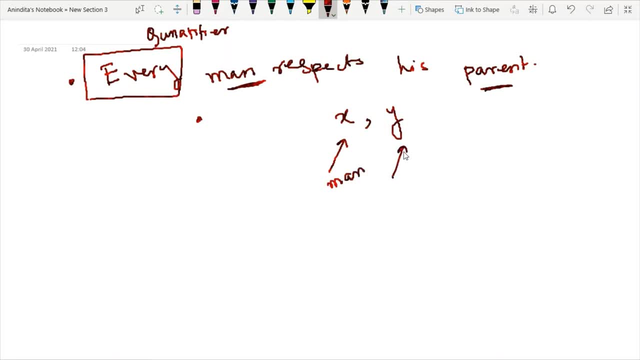 Here x is a variable. Which represents man. 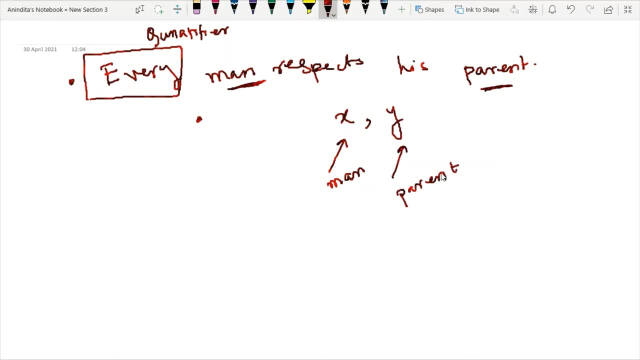 And y is another variable. Which represents parent. 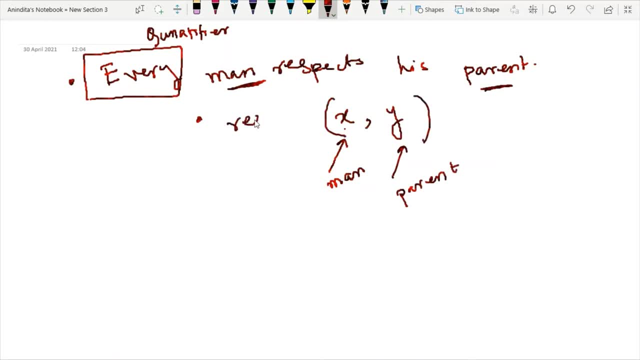 So in that case. x. Respect. Parent. 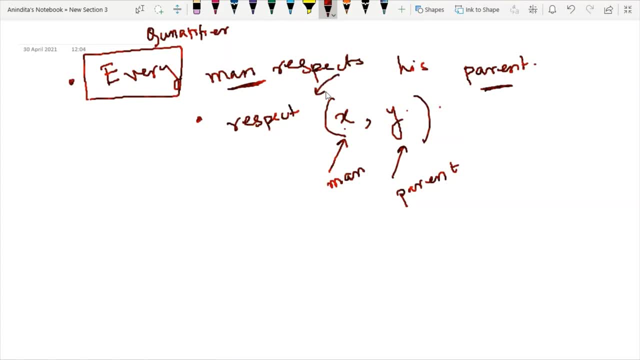 So this is my representation. Means the essence of this line. Now how could I represent it. 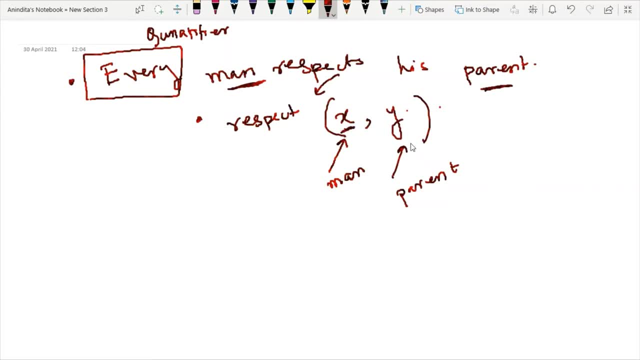 I know that. This person. 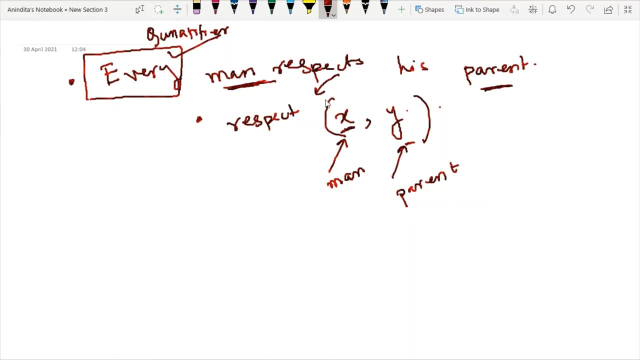 This variable. So every man. Means every x variable. 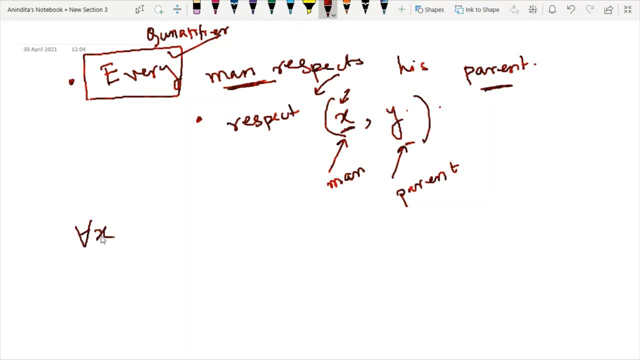 So for x variable. It is true. Okay fine. So for every we have this kind of representation. 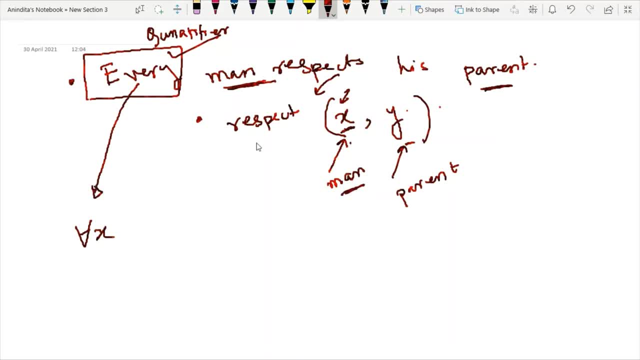 And since. X variable represents man. And we have written every man. 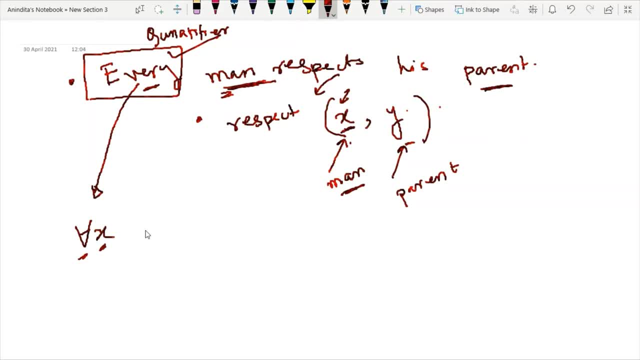 So I am written all x. Then the next question. 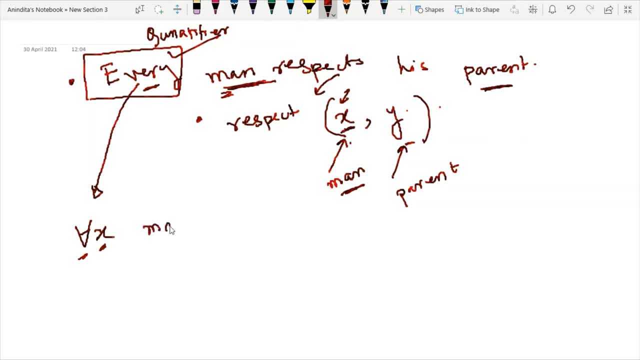 Will be who is x. So I have to write it. That x is a man. The elitist part is done. 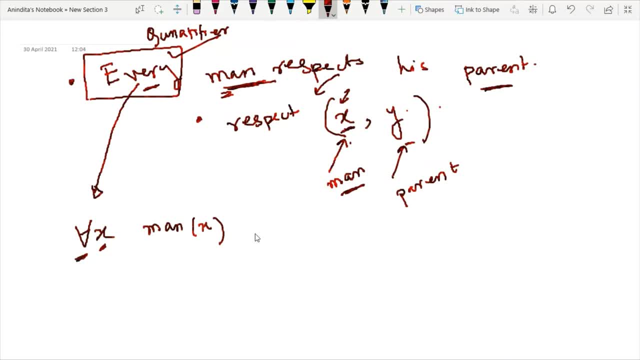 And what is the main connective. The main connective with all. Will be implication. And then. 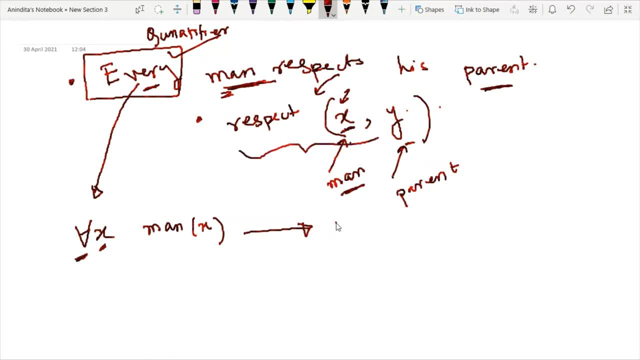 What is the actual essence of this line. That is respects. 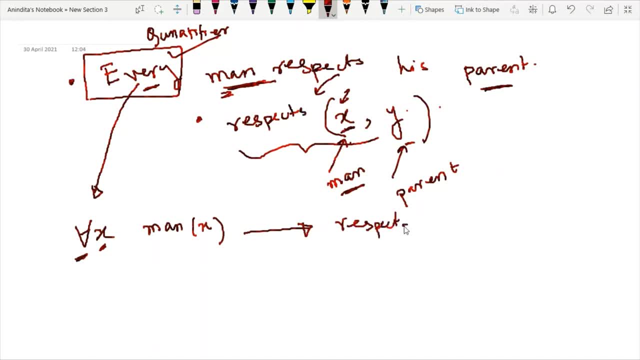 Respects. Or respect. Anything. 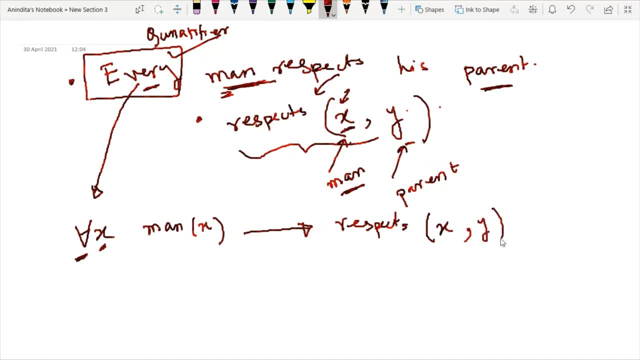 Who respects whom. X respects y. 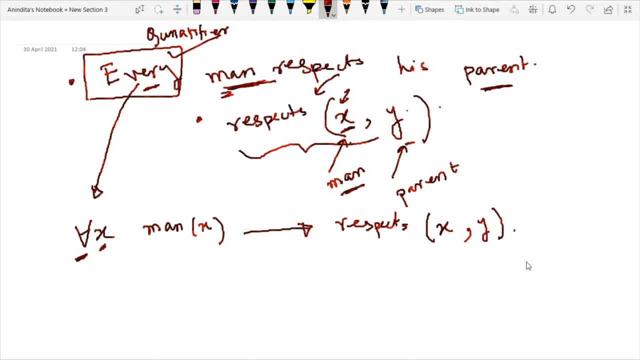 So this is another kind of. Representation. 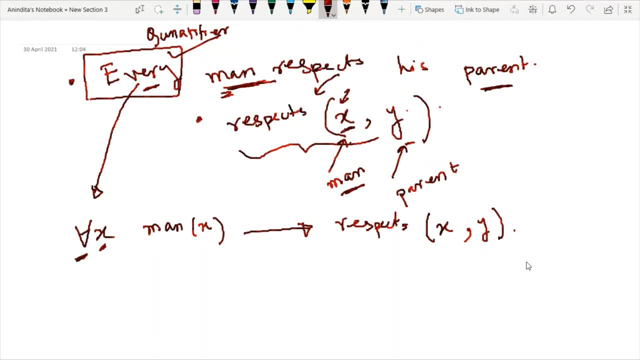 So first you have to identify. How many variables you have to use. So x is a variable. So means x represents man. And y is your parent. 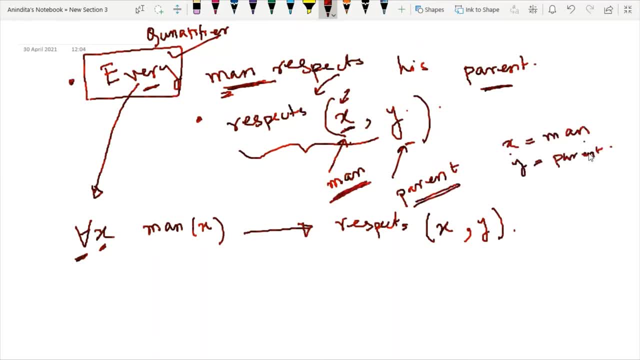 And y represents parent. Both cannot be same variable. 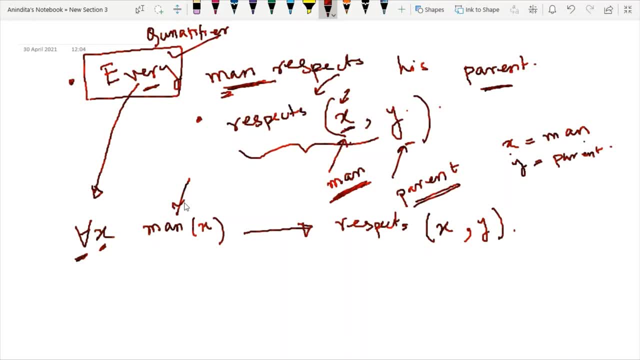 Now you may ask me one question. That you are stating that x is a man. But you are not stating that. Y is a parent. You haven't mentioned it. But you have used this y variable straight away. So here another trick is. 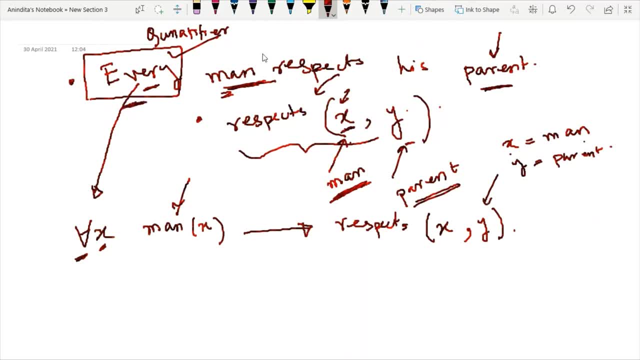 Whenever. Quantifier is there. With some variable. You have to define that variable. I haven't used any quantifier. With y. So for that purpose. If I write that y represent parent. Then it's fine. 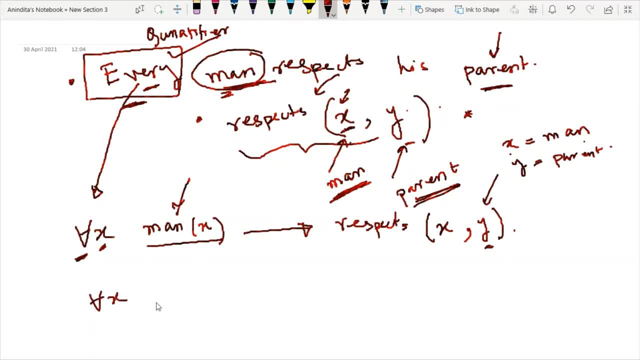 However this kind of representation. Seems very complex. 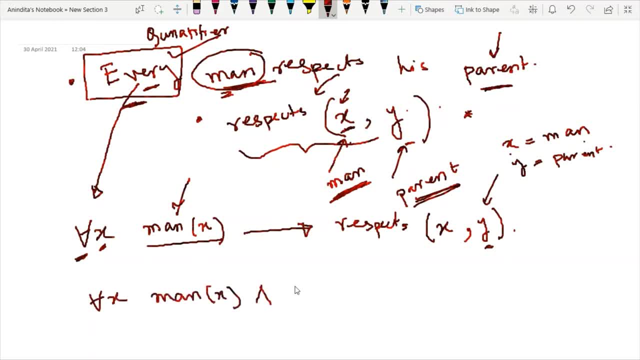 Because if you write for all x. X is a man. And. Parent y. Y is a parent. Then you can write. Respects x comma y. You can also use. This kind of. Representation. 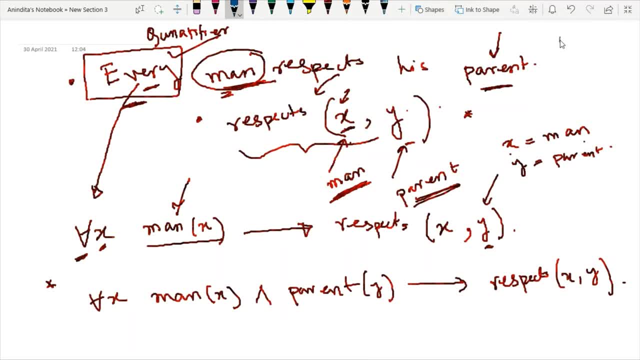 So now again. Try to understand. 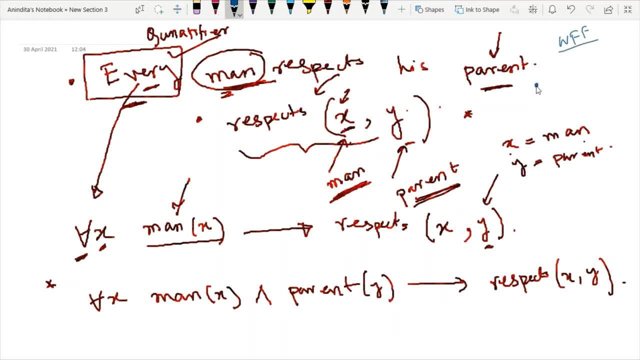 We are learning WFF representation. And also we have to remember. In WFF. Function within a function. 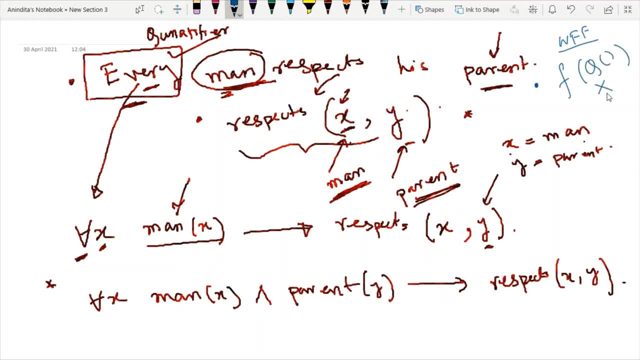 Is not allowed. Means it is not allowed. In first order predicate logic. So whenever you have. 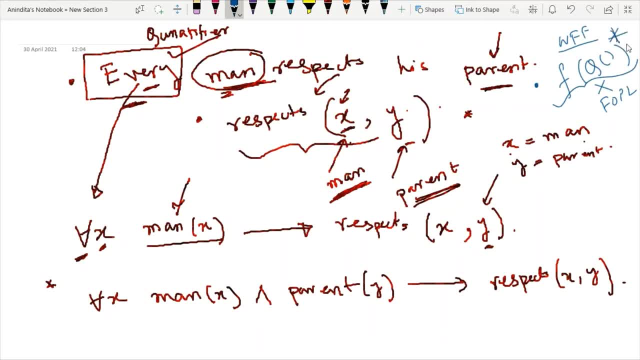 This kind of representation. It is not termed as WFF. 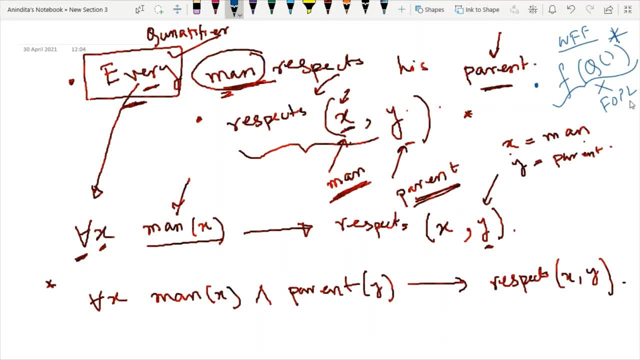 But. Along with this representation. Again there will be one question. 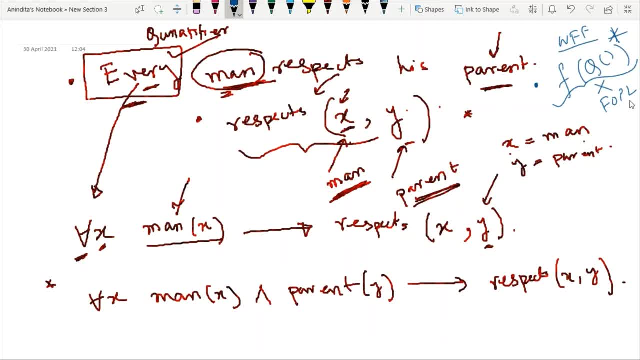 That how we can represent. The concept of not. Because. We cannot use not. Inside a function. 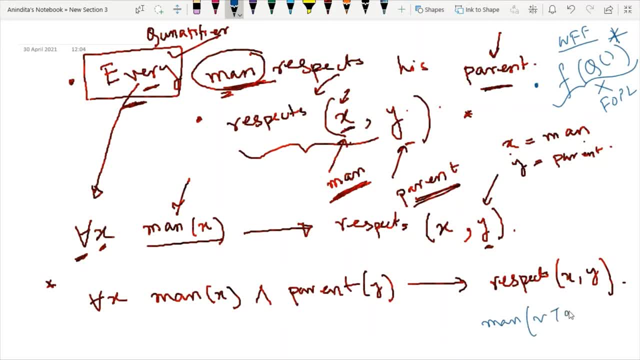 That is. Tom is not a man. 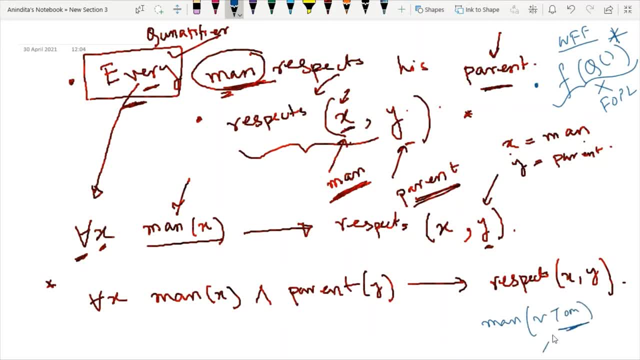 I cannot write. Not Tom. Inside a function. So now. Consider. 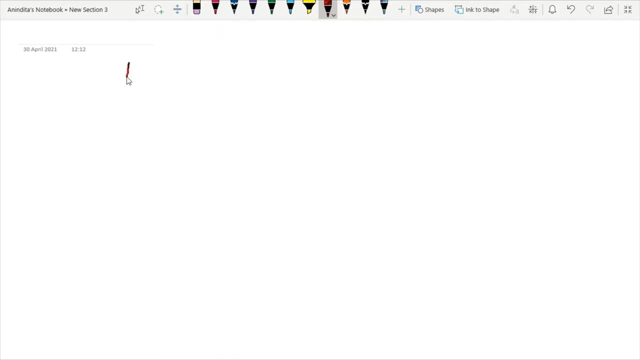 Another example. If the example is given as. 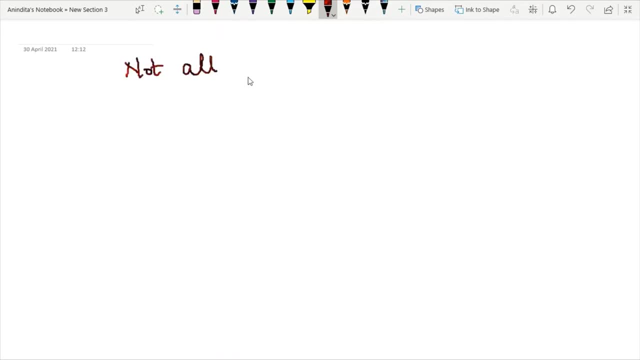 Not. All. Students. 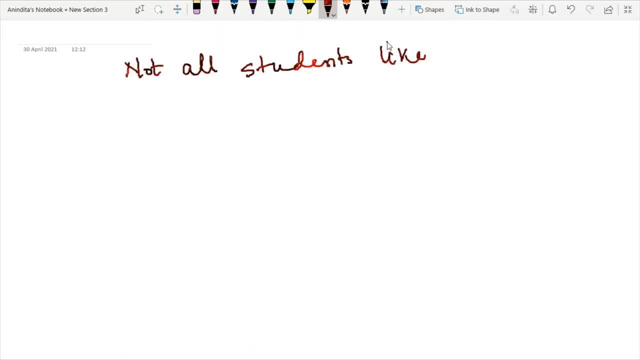 Like. Both. Mathematics. And. Science. So. Now. Let us. Say. This is my statement. 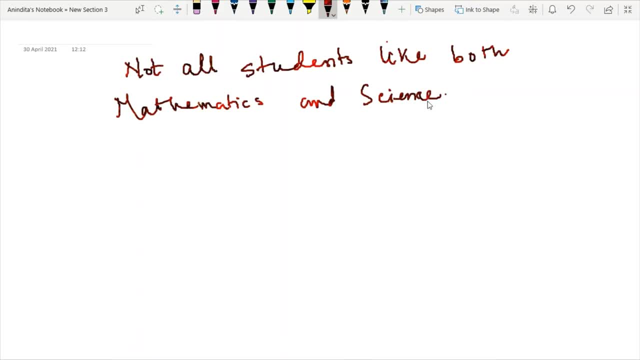 So in that case. We know that. We have to represent it. 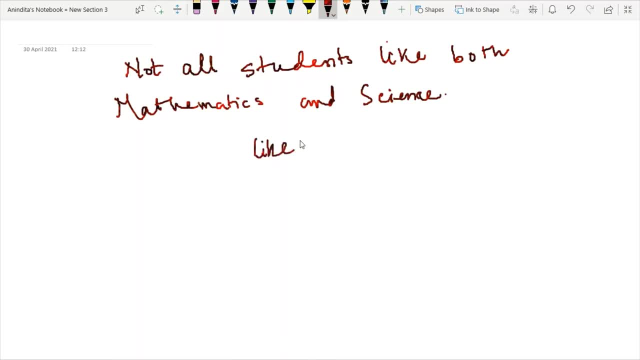 In terms of predicate. But what is the essence. 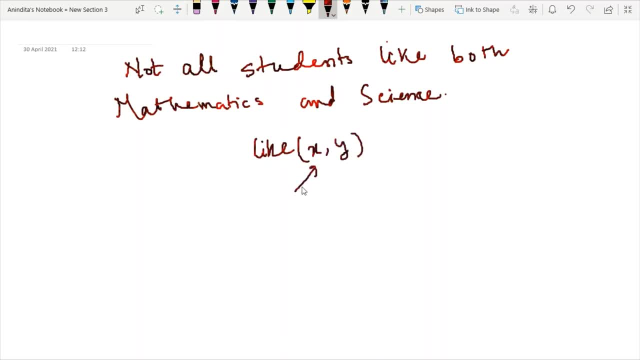 So basically I want to represent. Something like this. Like. 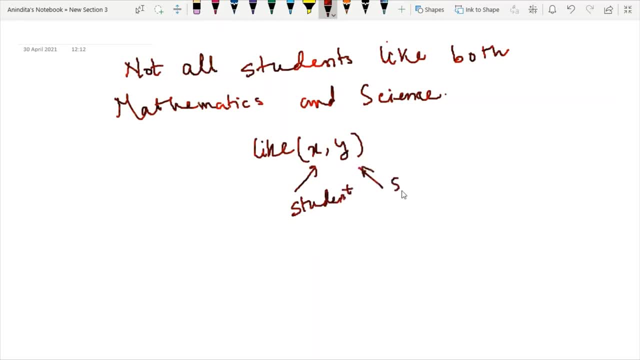 X,y. So what is x. 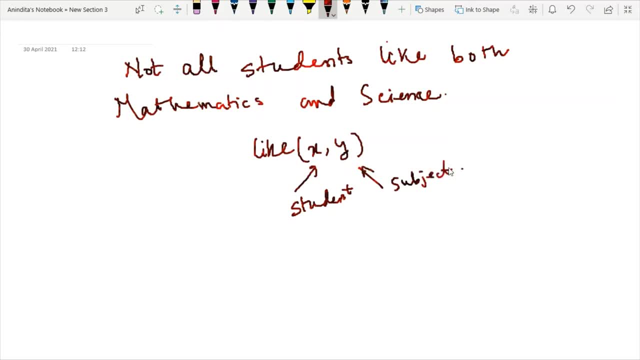 So I have to assume. X as student. 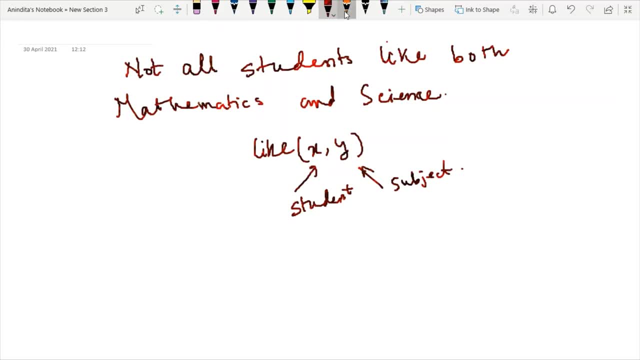 How we can represent it. So now we are. Getting one. Particular representation. Not all. 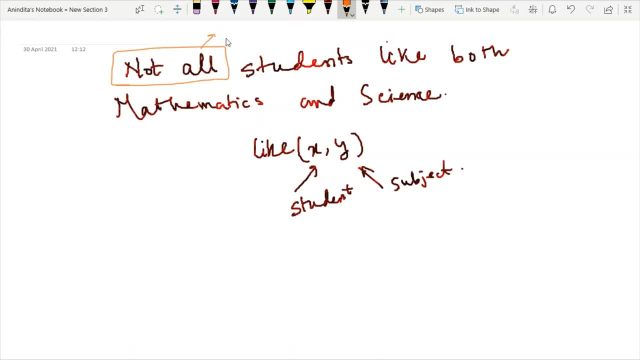 So in that case. The representation will be. We know that. 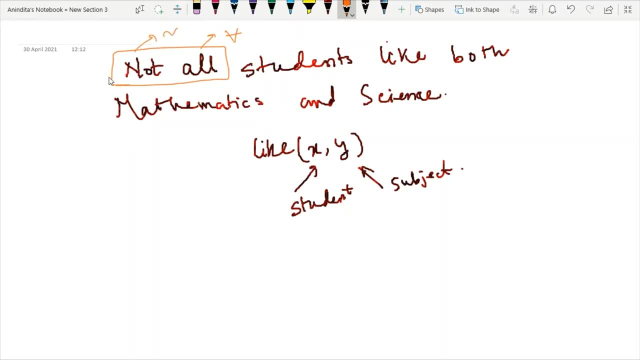 All means this one. Universal quantifier. 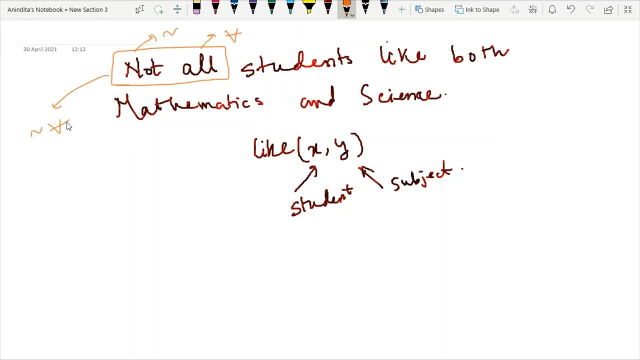 And not means this one. So basically not all will be represented as. 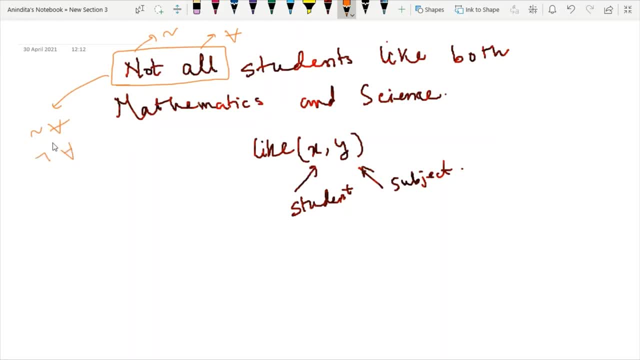 Not all. Or you can write it as not all. 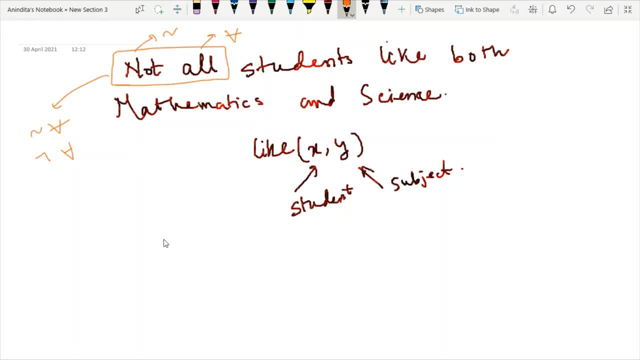 So in this case. Whenever you are going to write the statement. First you have to write. Not all. And we know that. Whenever we are writing any. Quantifiers. Then along with the quantifier. There should be one. 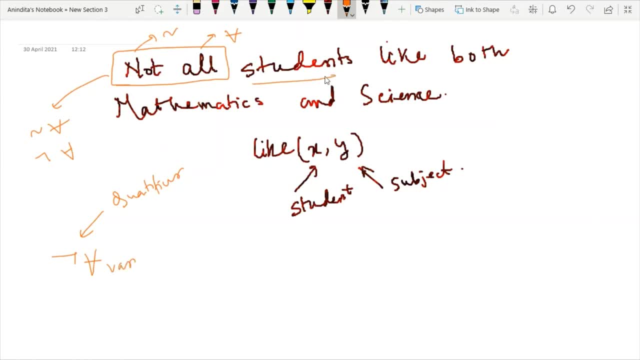 Variable. So what variable should I use. 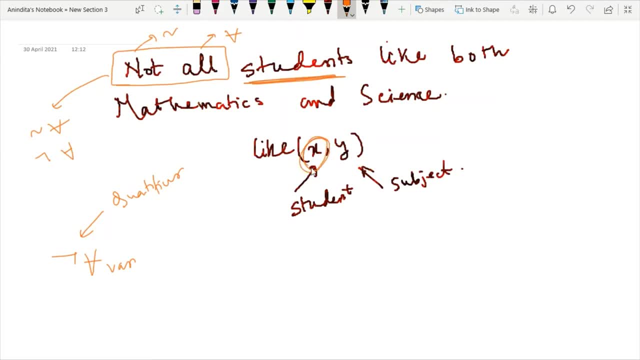 Not all students. So here student means. 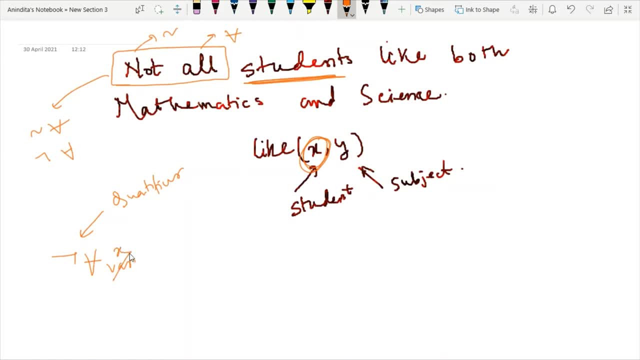 Variable x. So here I will write. And then. Definitely I have to state. Who is x. 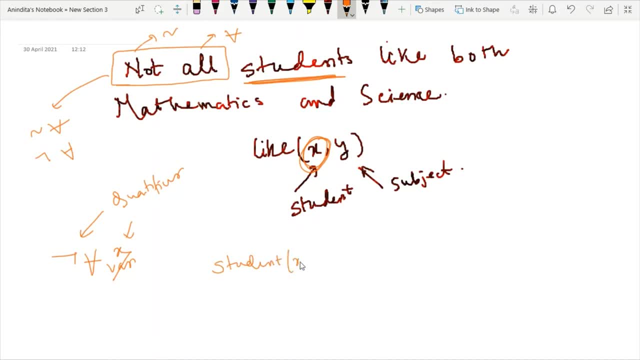 Then definitely I have to write. X is a student. So I will write student x. 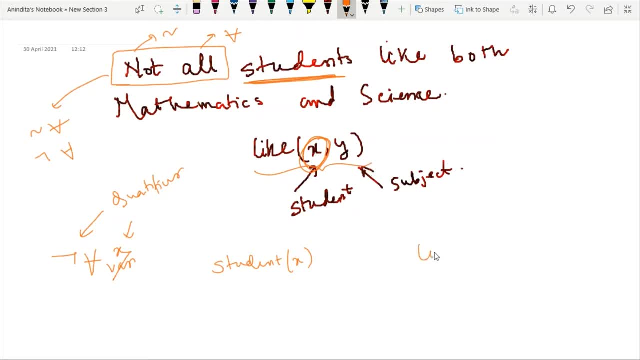 And then what is my. Representation. 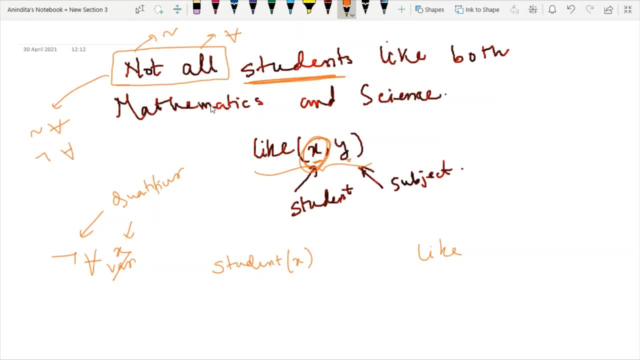 That is like. Not all student like. 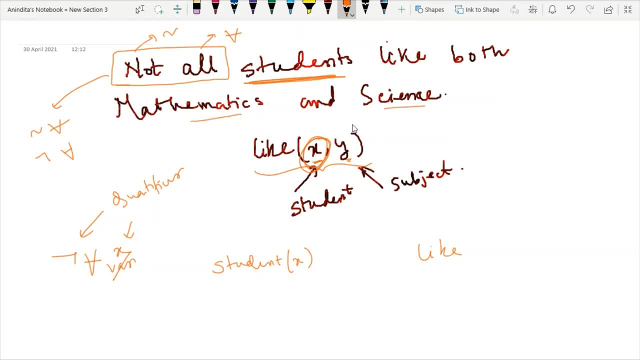 Mathematics and science. So here. 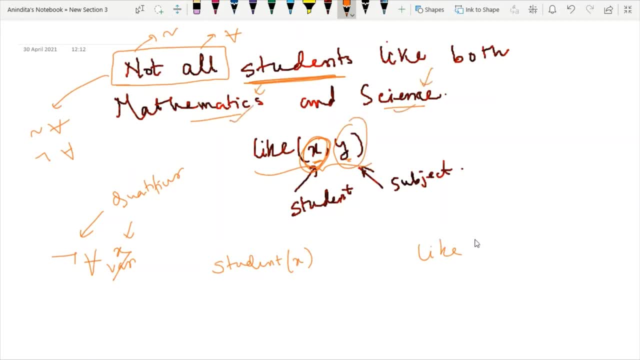 Subject name is specified. So I can write. Students. First. Subject name is here. 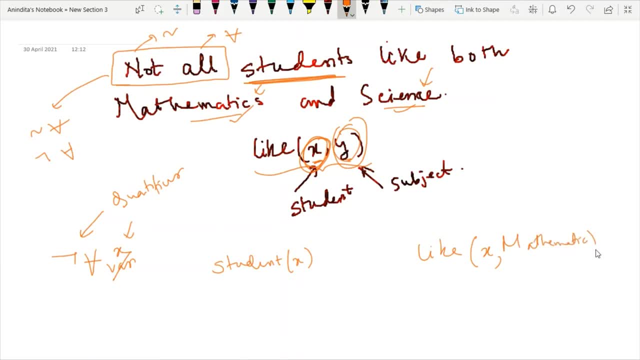 Y will be replaced by. Mathematics. 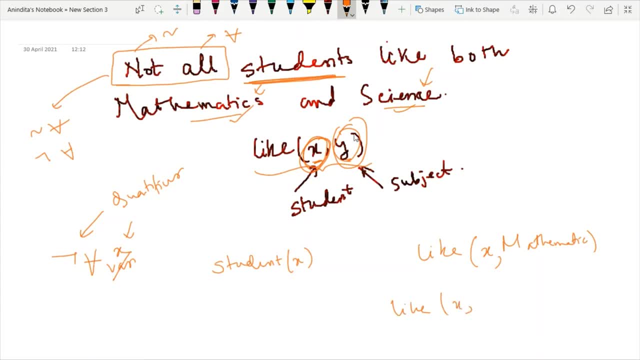 And the second thing. Instead of. Y I can write. 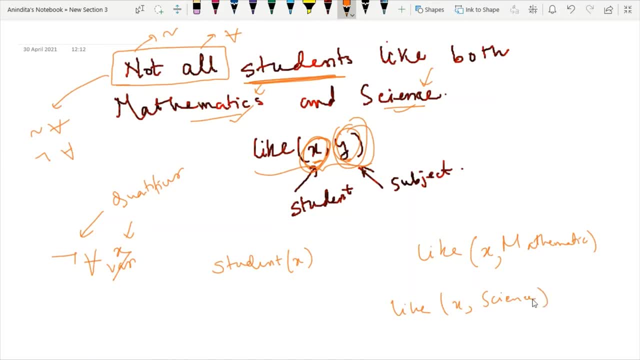 Science. So now how could I represent it. 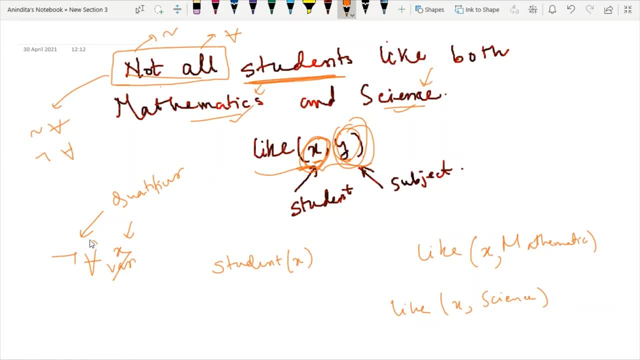 See not all. Student. Not all. Student. 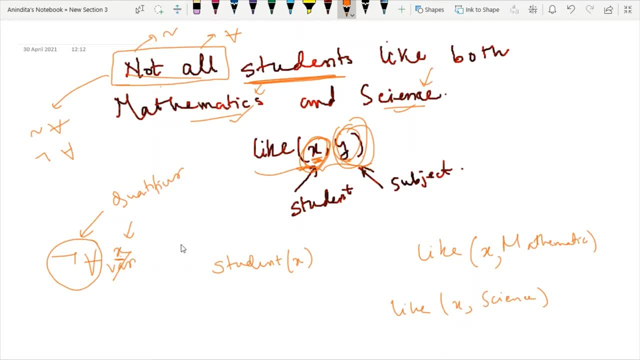 Here student means variable x. So I have written x. 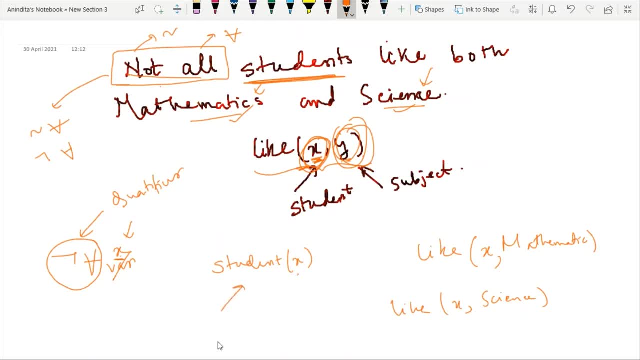 We have to define what is x. So x is a student. X is a student. 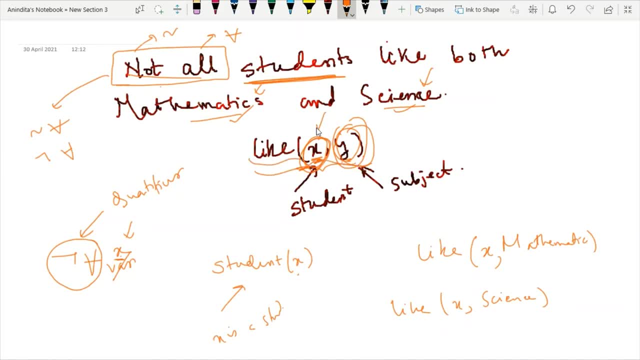 And what is the essence of the. Representation. 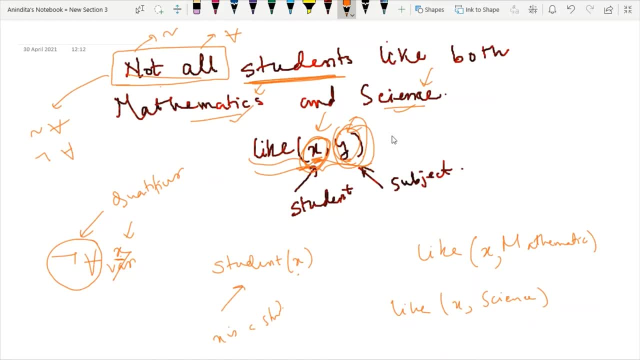 Student like mathematics. Student like science. 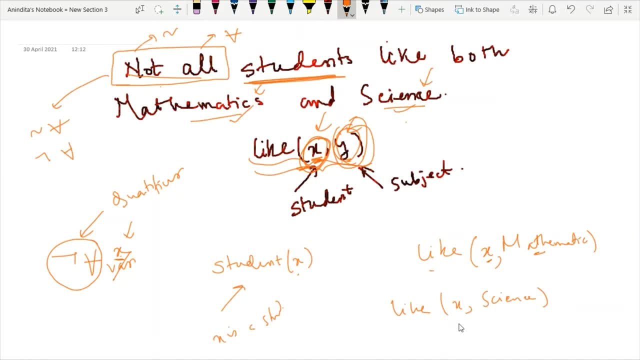 So like. Student mathematics. 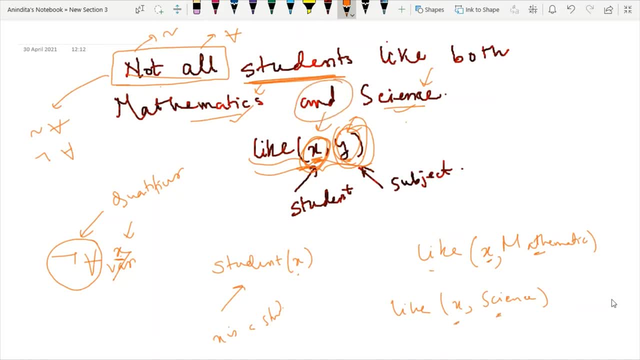 Student science. And we have and in between. 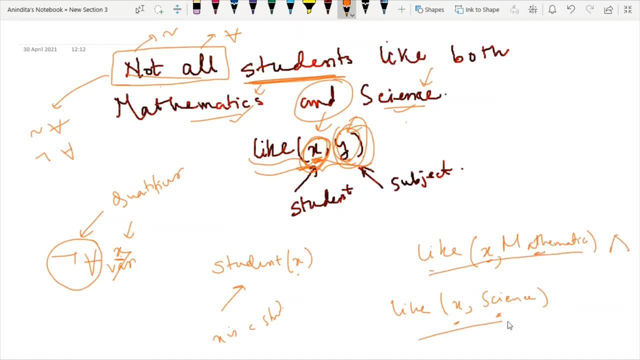 So in between two statement. This statement and this statement. 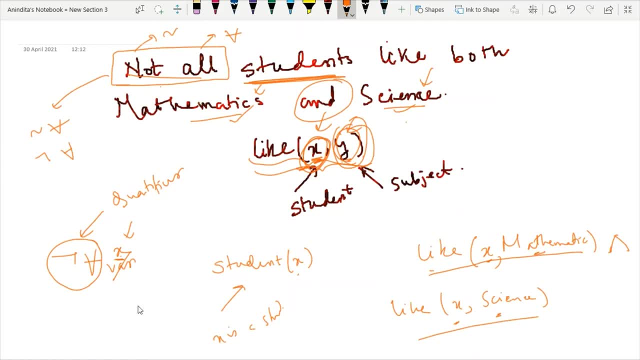 I am writing and. And we know that. We have this kind of representation. For all universal quantifier. The main connective. 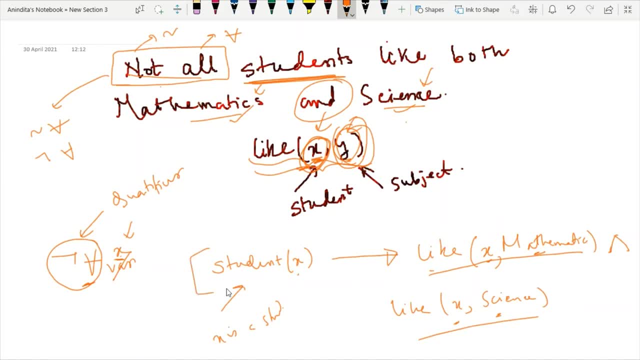 Will be implication sign. Now consider. 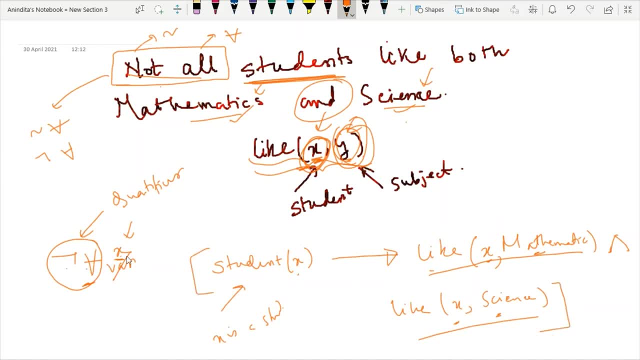 This statement the representation. Is over not all x. Where x is a student. Like mathematics. And science. So this is the representation. Now we have to learn. 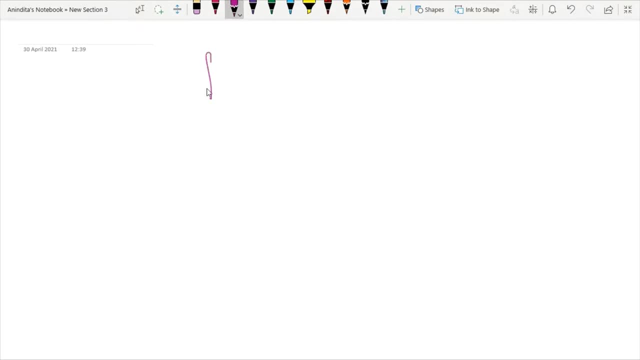 One simple. Definition. Of free variable. I am giving you. One representation. For all x. There exist. Y. P x comma. Y comma z. 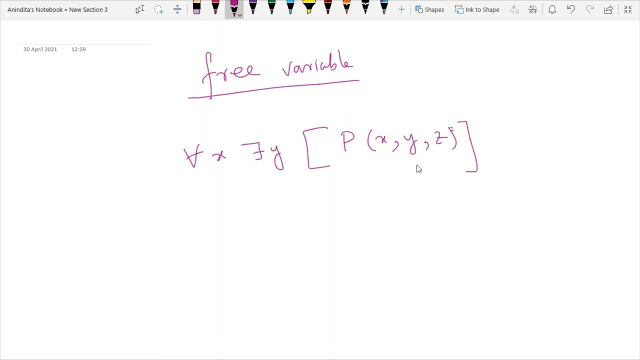 So this is my representation. The variable. Is said to be. Free variable. If in a formula. It occurs. Outside the scope. Of the quantifier. Try to understand. 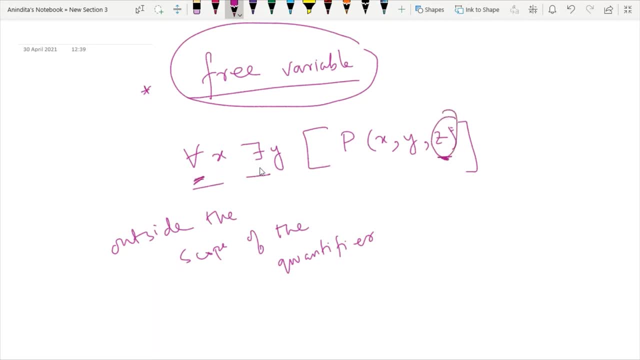 Here z exist. Outside the scope. Of the quantifier. The meaning is. With this quantifiers. We do not have the variable z. So that's why here. Z is termed as free variable. So definitely. Whenever. 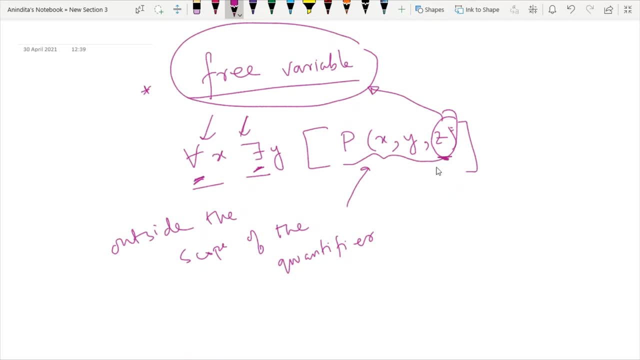 We have some specific function. Representation. 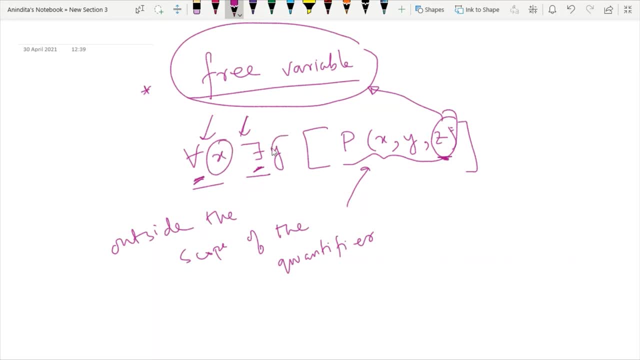 We may have more than two variables. However. They are represented. With the quantifiers. And when they are used. 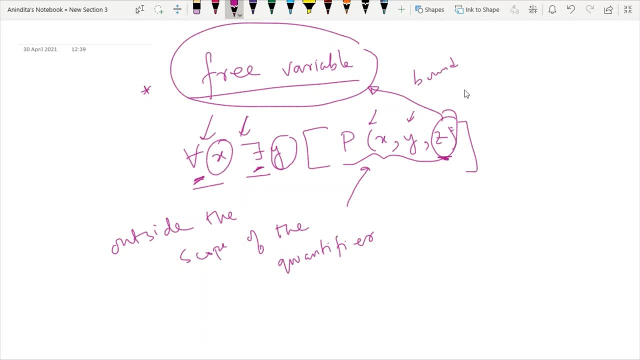 They are actually the bound variables. And the variable. Which is. Not used with the quantifier. 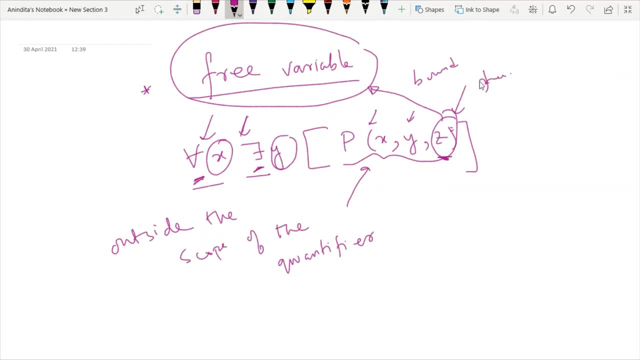 That is known as. Free variables. 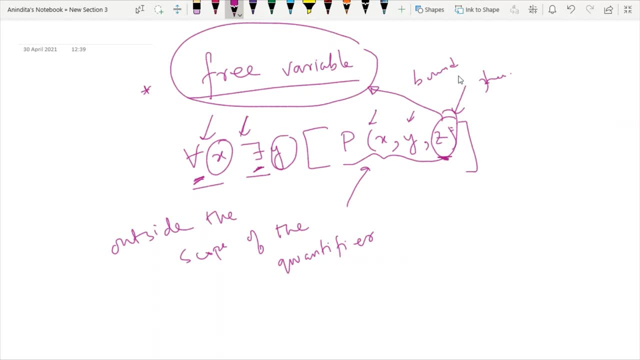 So while representation. Also in the advanced level. While representing. 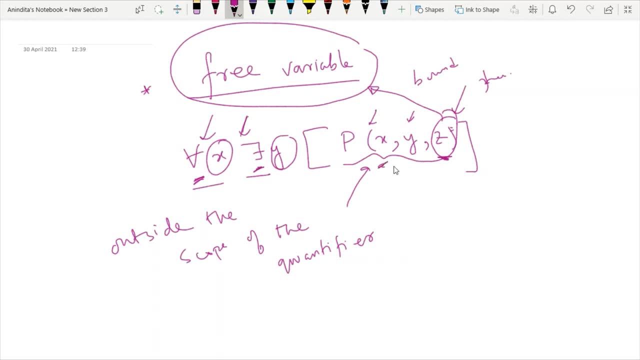 A particular English statement. We have to understand. 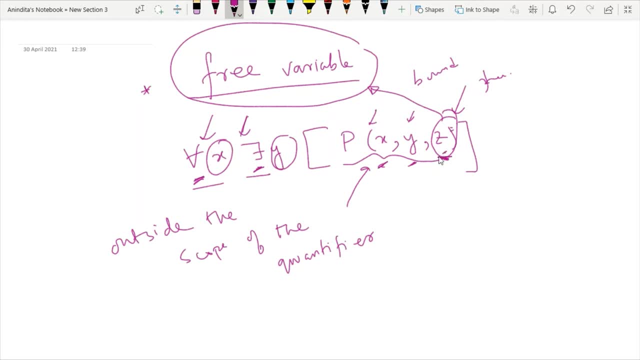 Which variables are bound variables. Are free variables. 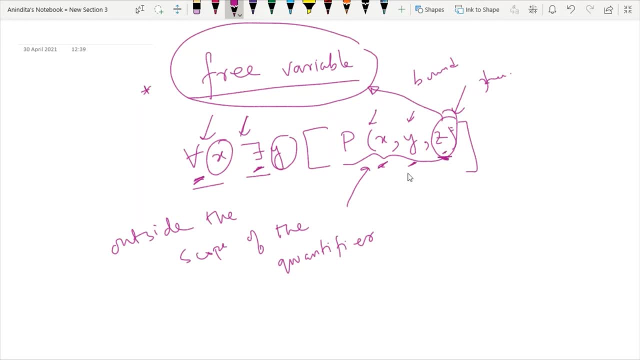 So what is the definition. Of a bound variable. 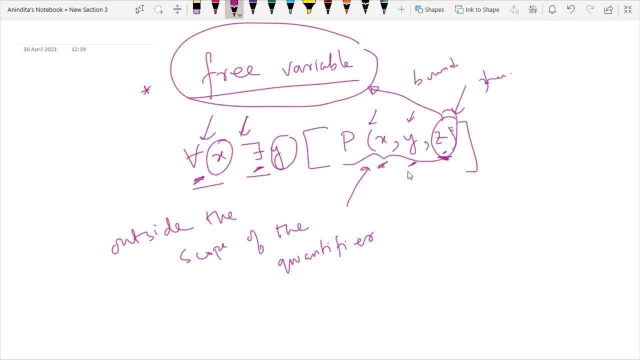 So definitely. I can say that bound variable. In a specific formula.